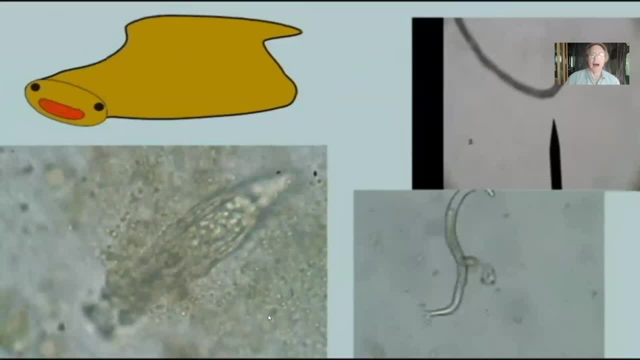 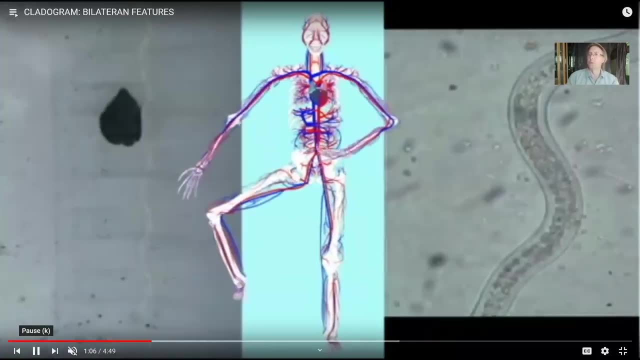 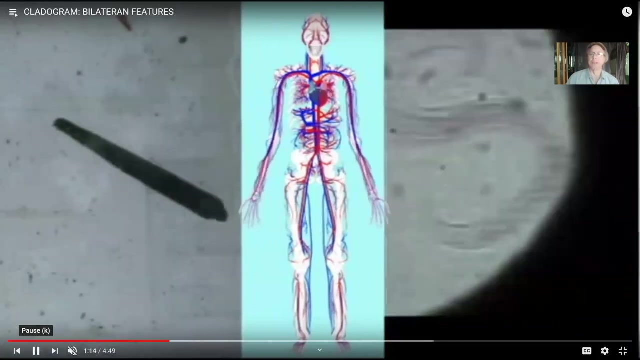 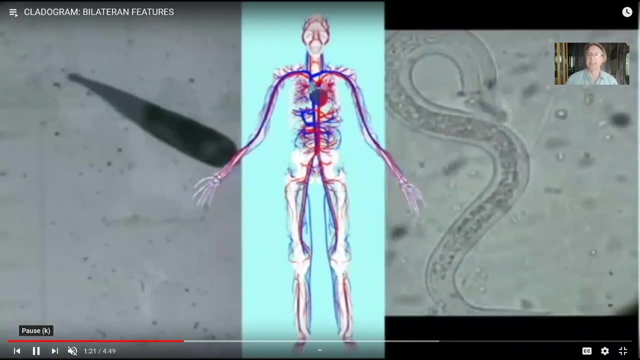 one could now invest more and make more complex eyes, And so this decision to now always go forward meant that an animal was no longer radially symmetrical, but now bilaterally symmetrical. The only way to cut an animal into two equal hands was to make left and right hands The bilaterally symmetrical. 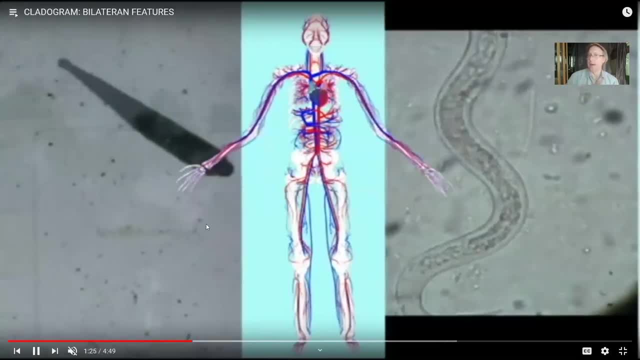 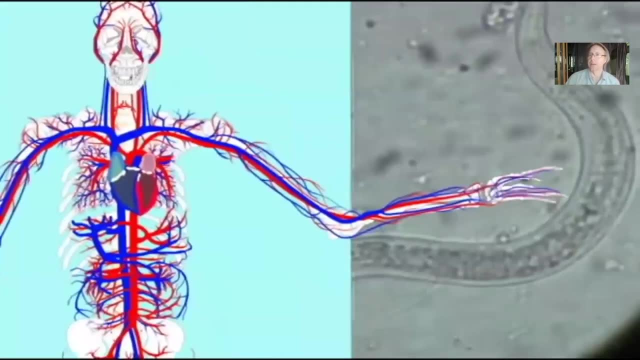 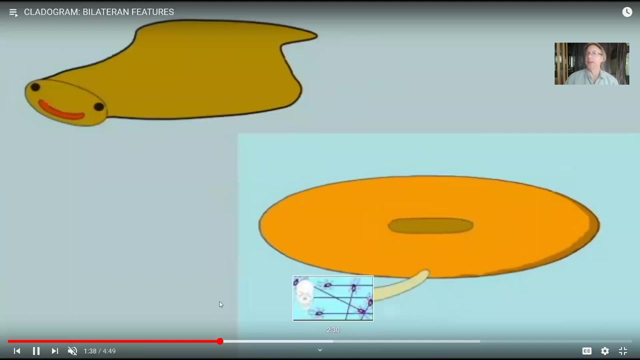 animals then share many other features. Not all of them have them, but, for example, blood vessels which is pumped by a heart- and a heart is really just contractile blood vessels- Changes in genes, a brain and a nerve cord- Now the original brains. 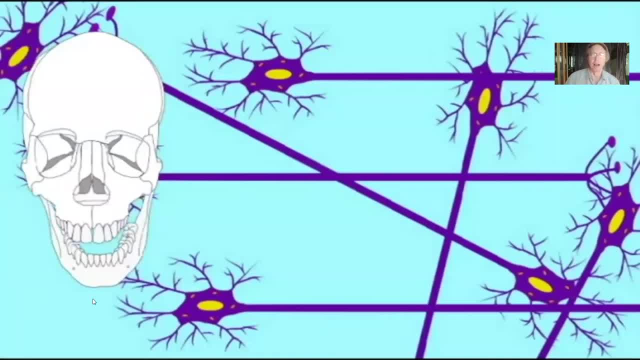 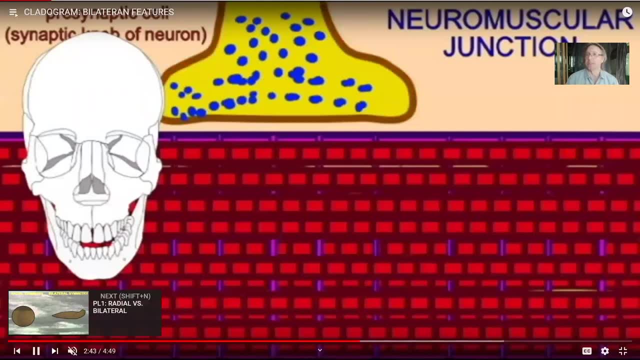 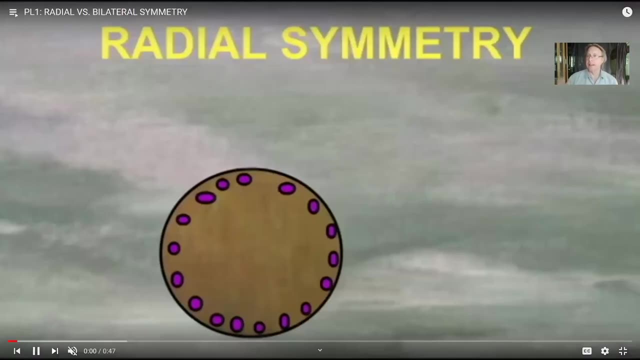 were not very complex at all, just a cluster of a couple of cells in the head region. Many would prefer not to use the brain when talking about the simplest of worms and use just the term, say cerebral ganglion. But once again, these animals, when they chose to no. 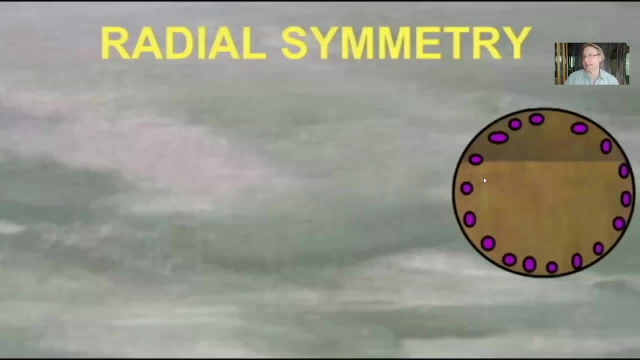 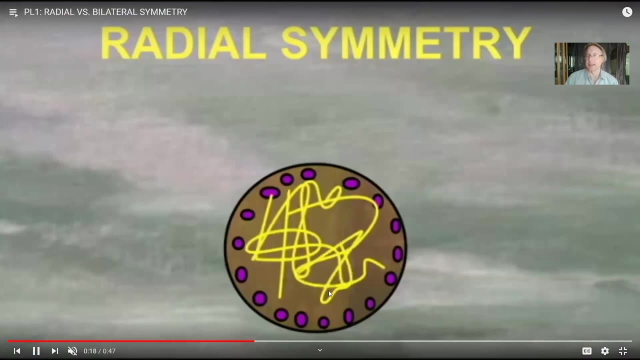 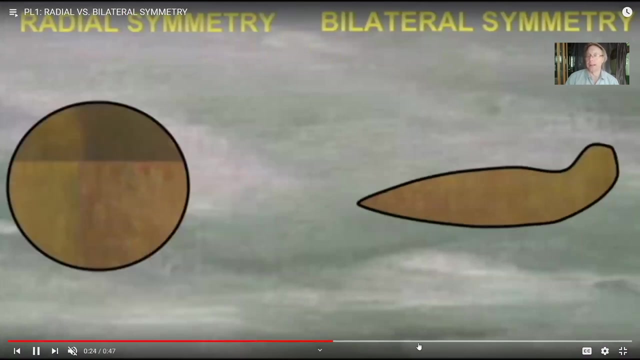 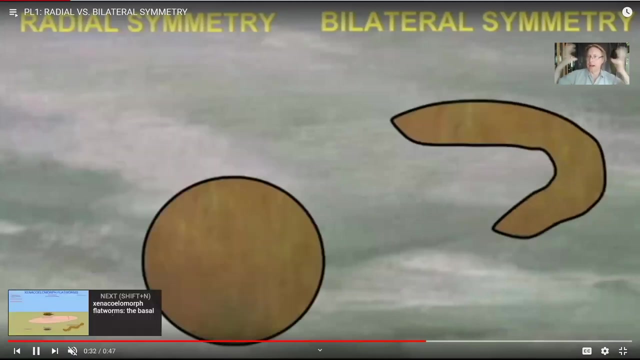 longer be radially symmetrical, as is this, say, Cnidarian with lots of those small eyes and a nerve net. This nerve net would be equally distributed, And any animal which is going to always go forward with the same body part first is then now more likely to develop a cluster. 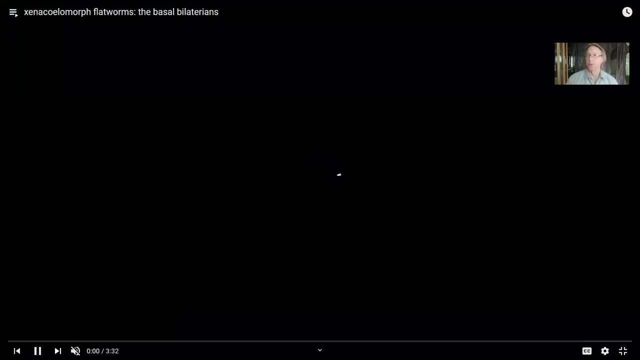 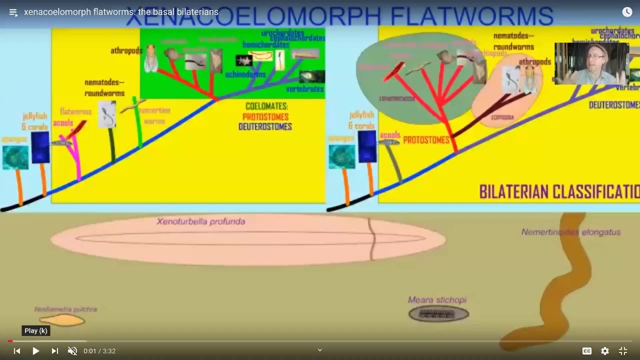 of sensory structures at the head end and thus the neural tissue, to process all of this sensory information. Now this video is being made for students who want to get an overview of the brain, So I'm going to move quickly into the next video, which will have the arthropods And 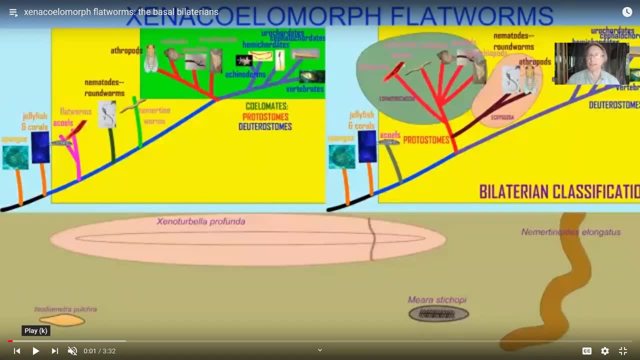 so getting bogged down in all of the classes of modern worms is a little bit beyond the scope, But I would like to mention a couple of points. So here there are a couple of modern representatives of what are called the Xenocelomorph flatworms. 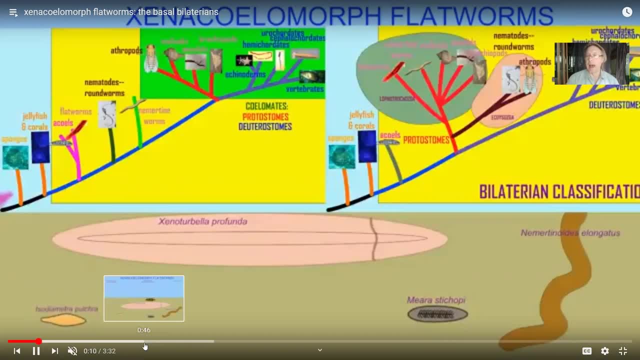 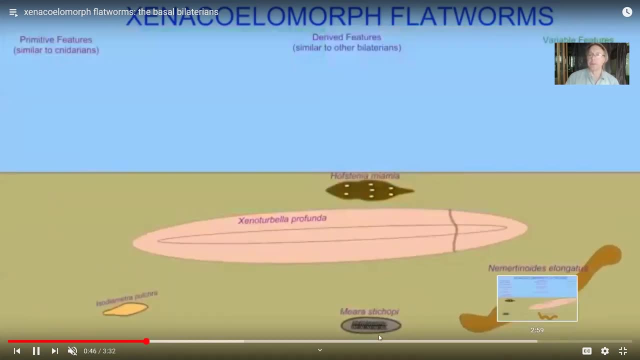 They are the most primitive bilaterally-selected. They are the most primitive bilaterally-selected. They are the most primitive bilaterally-selected. They are the most primitive bilaterally-symmetrical animals and therefore are good models of what the first bilaterians might look like. 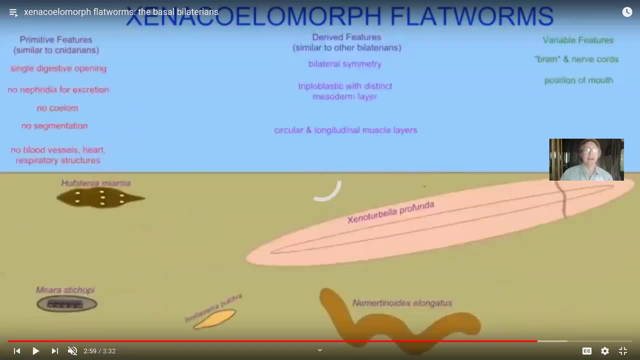 And so these are alive today And they have primitive features which remind us of Neidarians and are more primitive than all other bilaterally-symmetric animals. So, as I'll go through, they have a single digestive ovum opening. They don't have any excretory structures, They have no body cavity or coelom. They are not segmented. They don't have blood vessels or heart or respiratory structures. They are more advanced than cnidarians because they don't have bilateral symmetry. They do have a third tissue layer of mesoderm. They possess circular and longitudinal muscle layers And 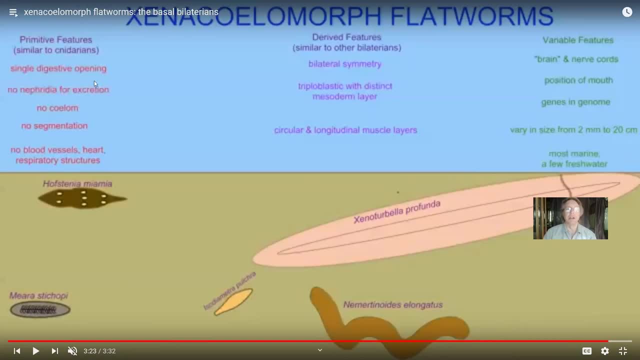 there are a couple of things which vary. So the position of the mouth can be more towards the head end, somewhere in the middle, or it can actually be in the center of the body, The size, the habitat, how large the brain is, whether there's actually a collection of neural cells. 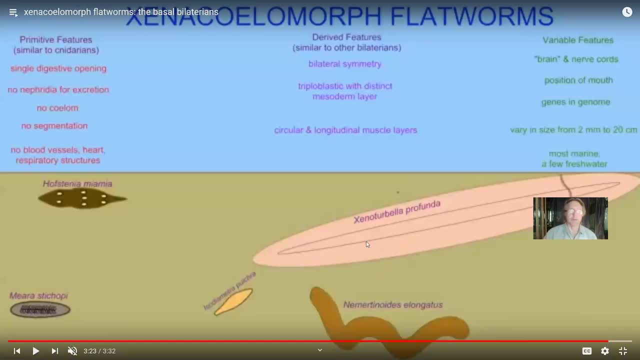 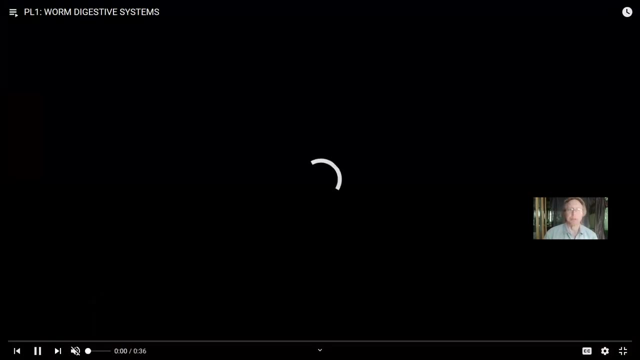 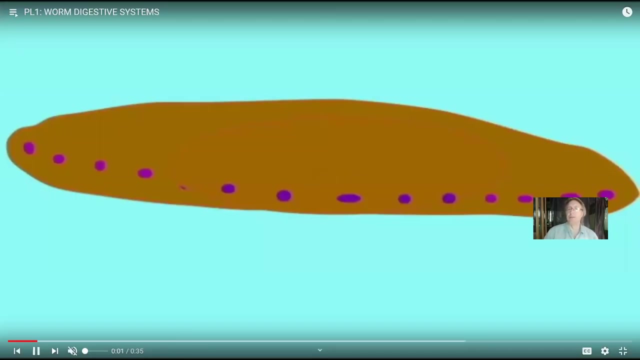 So because there's some variation, trying to piece together what the very first members of this group look like can't be established For certain. Now it is significant that cnidarians have a mouth in the center of the body and that these most primitive flatworms have a mouth in the center of the body. So even after 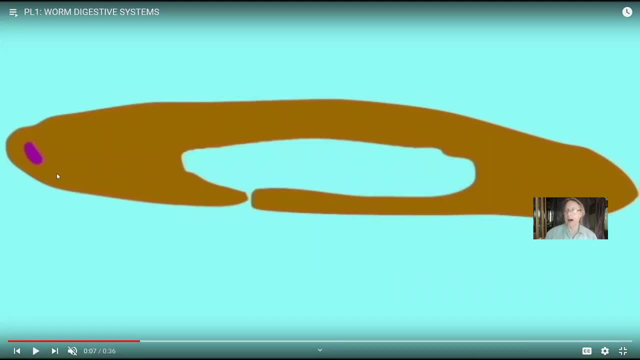 a head has been created- the mouth did not necessarily go there, And so sometimes it was center of the body, Sometimes it was closer to the head, but not actually at the head yet- And notice that there is one digestion, There is one digestive opening. So food would come in through this opening, It would be digested here. 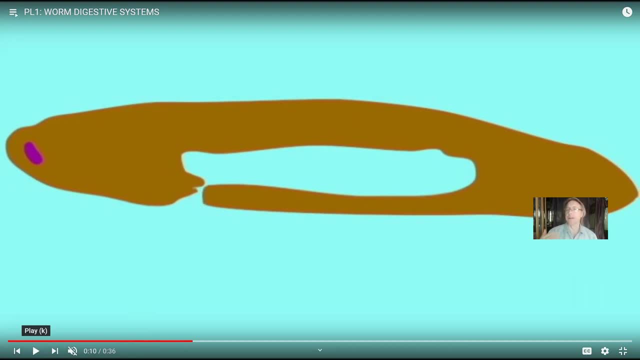 And then waste would be excreted through the same opening. So there was an incomplete digestive tract. It would only be in the more advanced worms that the mouth would move all the way to the head end And that instead of having a single opening, then the digestive tract would have an anal opening. 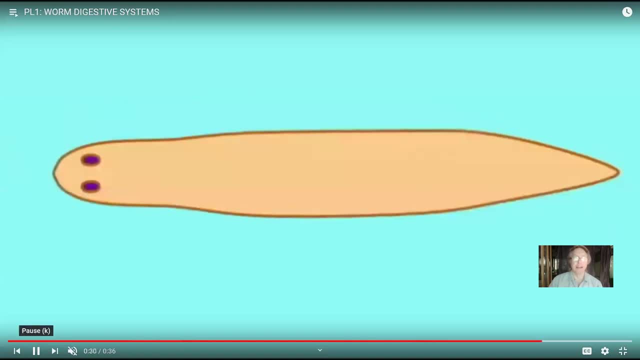 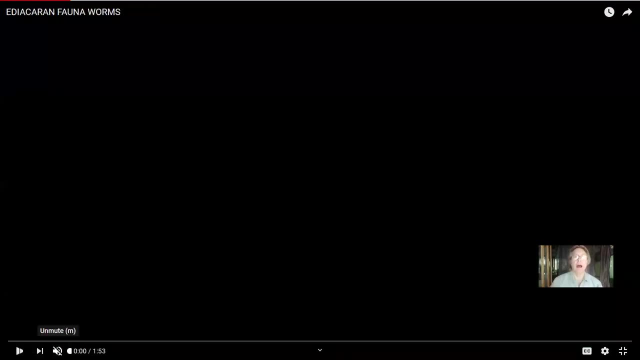 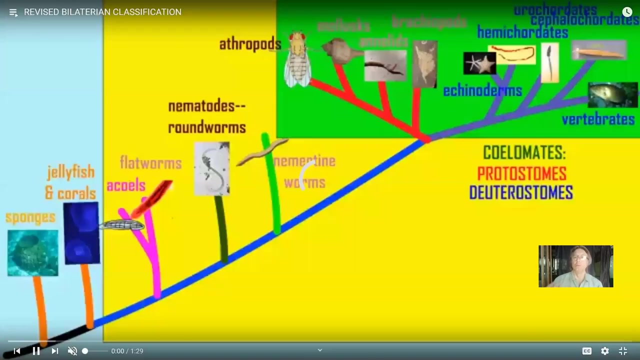 as well. This would be what's called a complete digestive tract. Now, this had appeared by the Ediacaran period, because there are burrows. There are not only fossils which are worms in the Ediacaran period, There are burrows of worms. 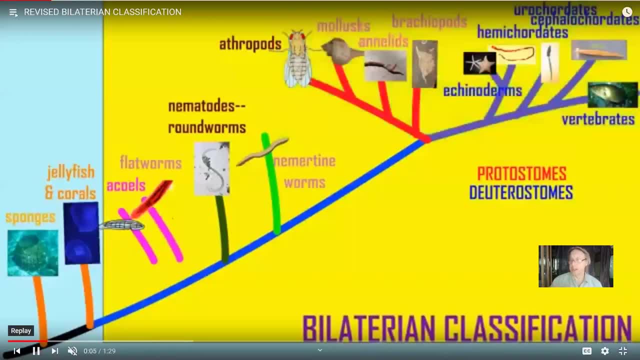 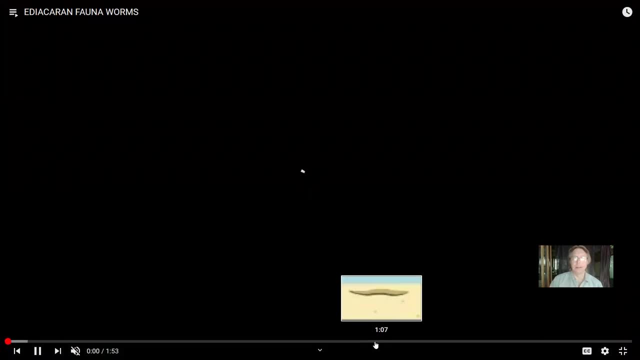 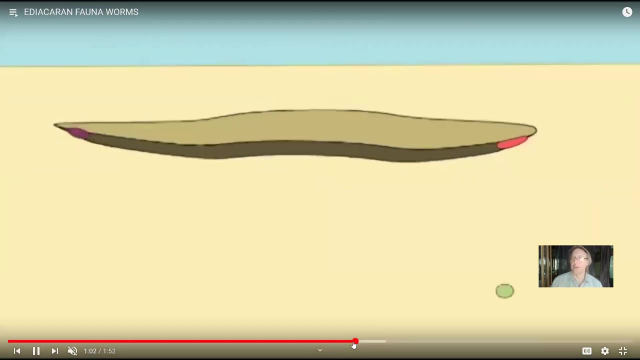 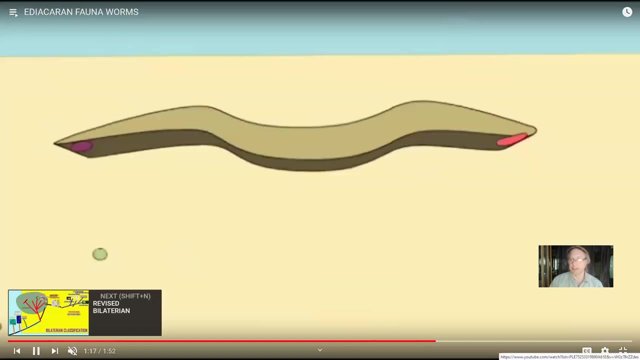 And then there are also burrows which have fecal pellets which seem to suggest the existence of complete digestive tracts, And so That during the Ediacaran period, not only did the primitive animals take that next step to the bilaterally symmetrical forms which had organs, which had a brain, but also then into a higher scenario where instead of an incomplete digestive tract, they had a complete digestive tract. 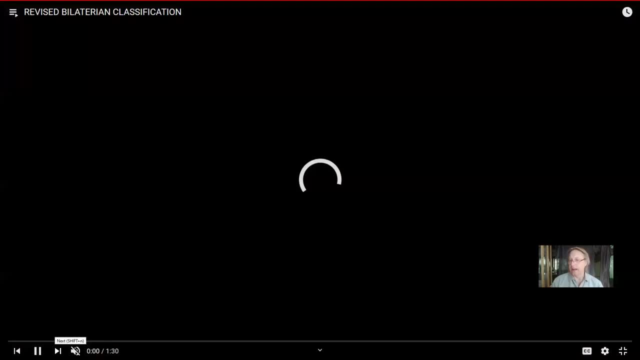 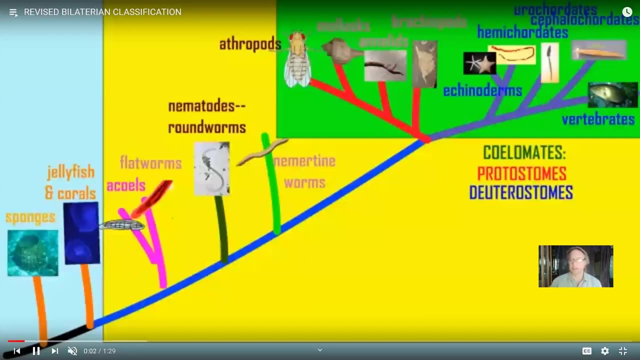 Now, after that, it gets a little bit more complicated. And I just mentioned this, you know, just so that you know, biology students are able to understand this And biology students are introduced to this idea, but not with the idea of those concentrated on fossil. 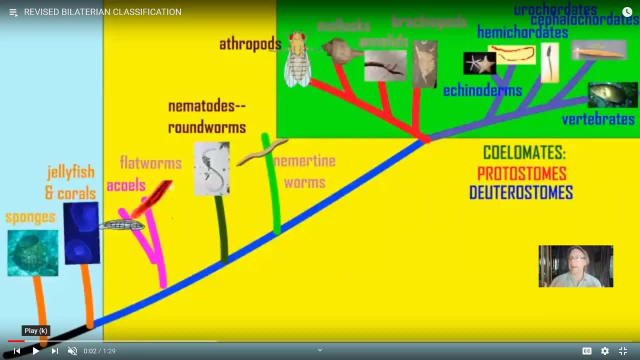 invertebrates need focus on this. for long, It was previously thought, for example when I was in school, that things like planaria and flatworms of today were with those Xenocelum morph flatworms as being very primitive, Because these flatworms, for example, do not have segmentation. 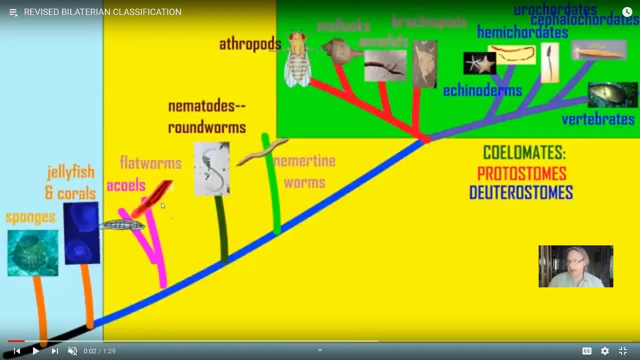 They do not have blood vessels or a heart and their heart is in the middle of the body. These worms, nematodes, which are primarily microscopic, were thought to be a little bit more advanced, Nematine worms. a little more advanced, they actually had blood vessels. and then it was thought that these animals that have a coelom, a body cavity, and also which typically have a circulatory system, that these would form a group. 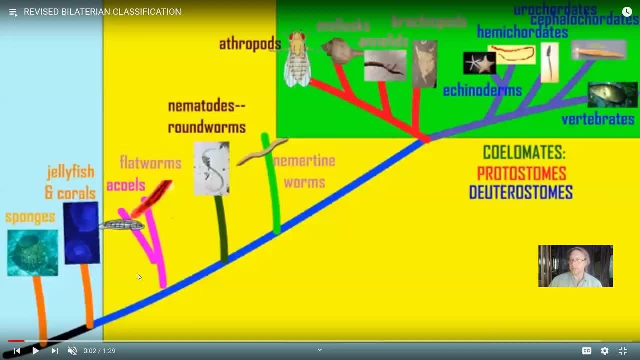 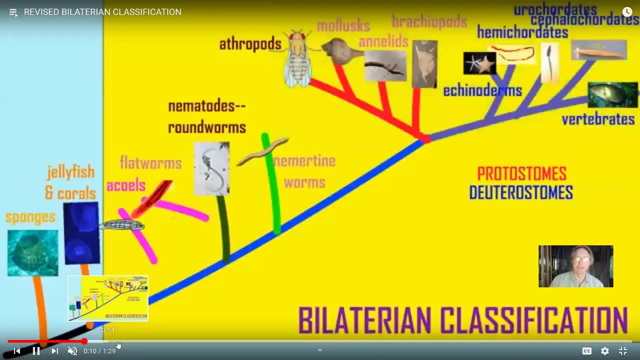 And so that the evolution of more complex bilaterin- or, I'm sorry, bilaterian- groups occurred in this fashion. That organization was primarily based on anatomical traits. Now that we can compare genes, genes sometimes suggest a slightly different branching pattern of the family tree than anatomical traits. 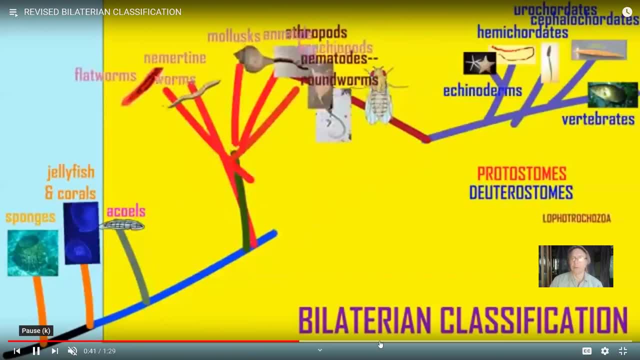 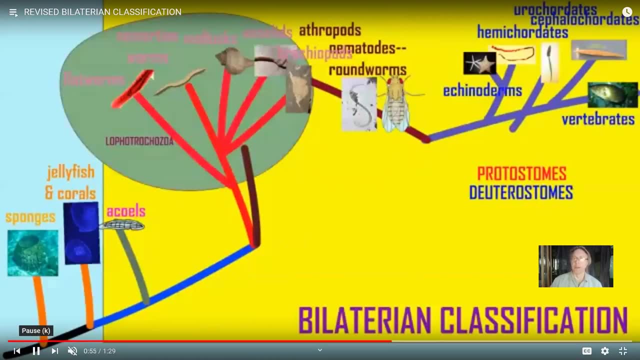 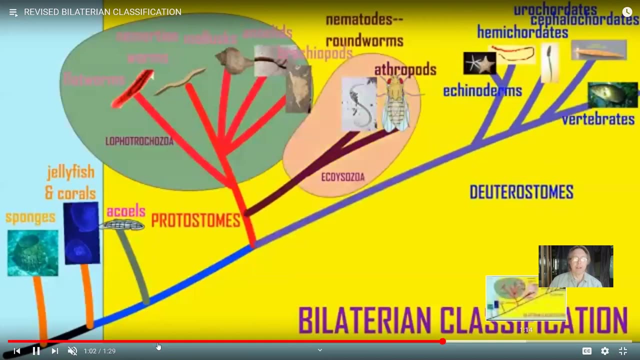 So we're going to go back to the gene that we're used to. So, therefore, what genes seem to suggest and what biologists are fairly comfortable with- although there are some unresolved issues which I'll get to- is that the classification would look something like this: 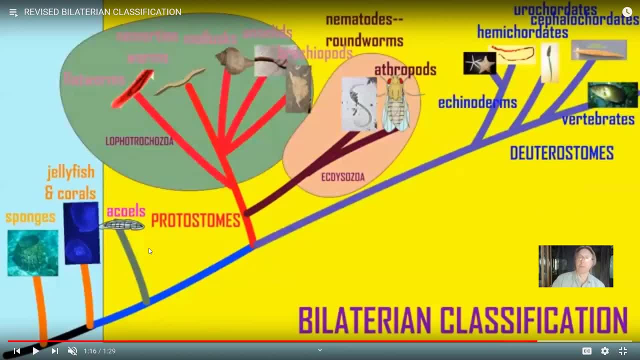 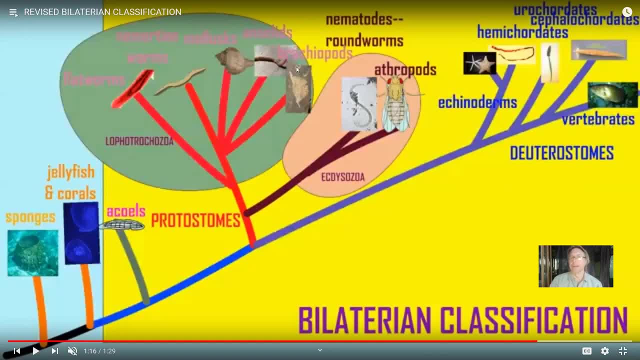 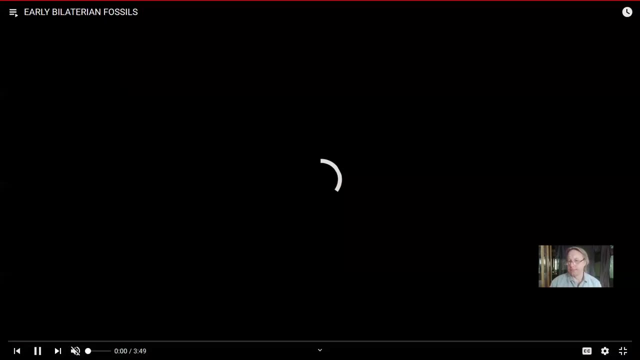 genes seem to have a lot of potential. lump them in this group, you know, together with a segmented annelid. worms and mollusks and nematodes, rather than being intermediate, would now group here with arthropods, And so there are two different models. Now the problem which I have, you know once again. 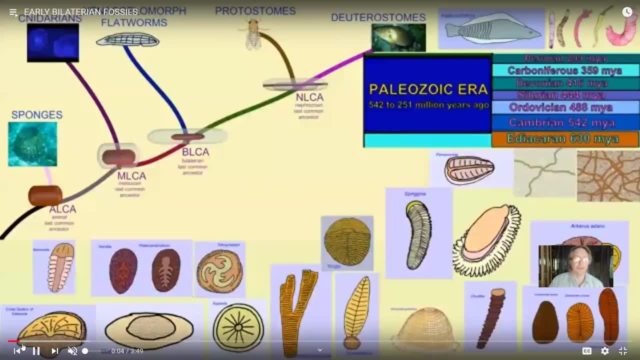 I'm a little older and then so perhaps I, you know, because of being, you know, stubborn, you know, prefer the older way. The problem, then, is if you were going to try to ask, all right, what steps in evolution occurred. So let's go with the revised classification. So animals 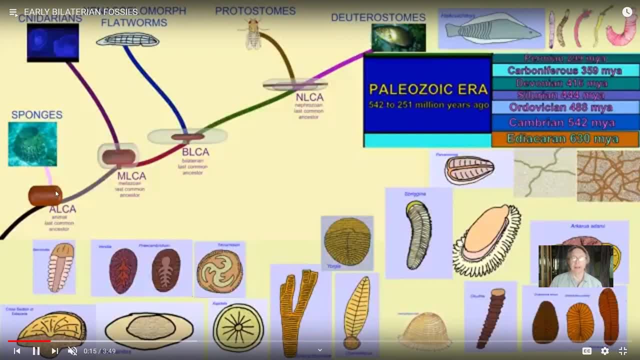 so evolved prior to the Ediacaran period, And so we think that the animal, last common ancestor, the organism which was the ancestor of all animals, would have occurred by the Ediacaran and perhaps a little before. There are, you know, sponge fossils, you know, which seem to be prior to that, Since the Ediacaran. 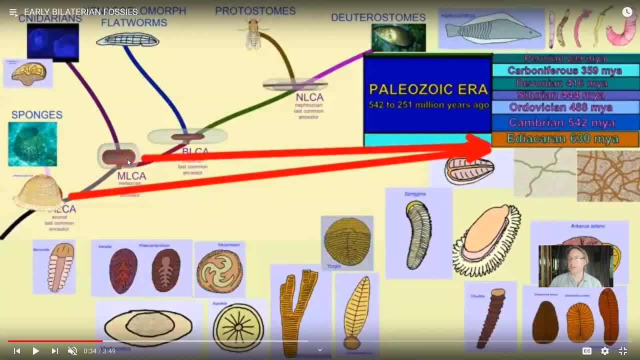 fossils are predominantly Cnidarians, then certainly the last common ancestor of the Cnidarians and the higher animals, the metazoans would have occurred by the Ediacaran, Because there are worms in the Ediacaran period. then certainly the last common ancestor of all of. 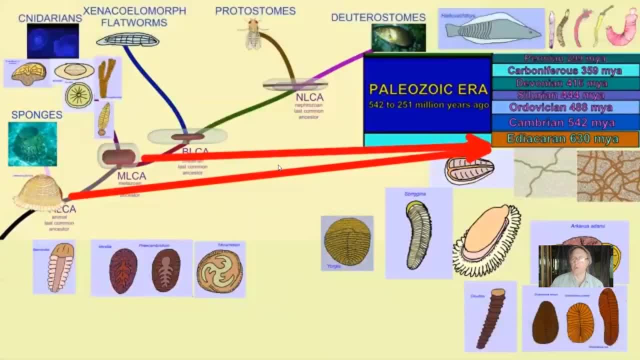 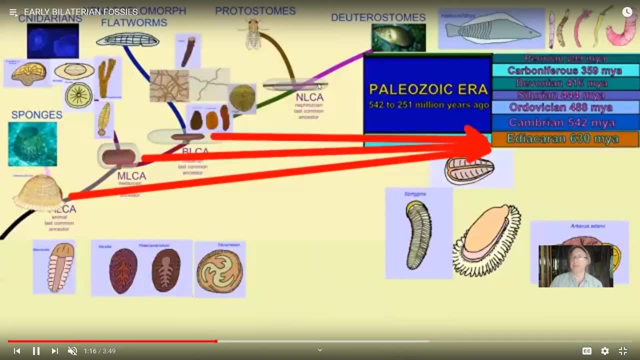 the bilaterally symmetrical organisms would have occurred in the Ediacaran period And because there seem to be higher animals by the end of the Ediacaran period, more complex worms with complete digestive systems and then transitional worms. then there is a lot of more complex worms. 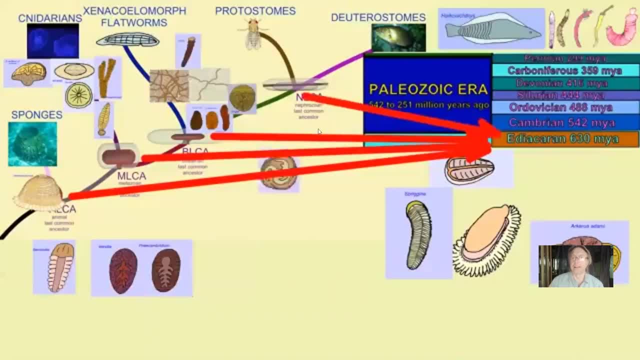 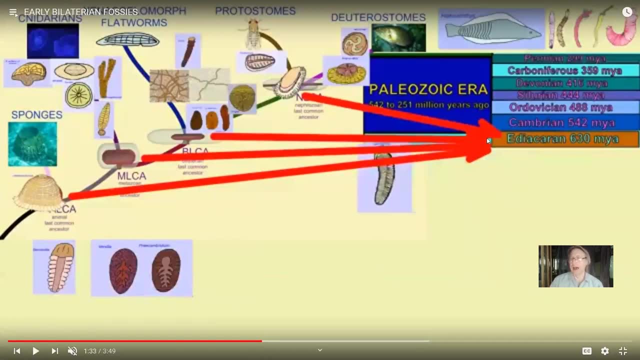 forms partway on the way to mollusks, arthropods and echinoderms. So it would seem that in the family tree of the bilaterally symmetrical animals, that a lot of things happened in the Ediacaran period by the end, And so by the time that the Cambrian came around, there were already 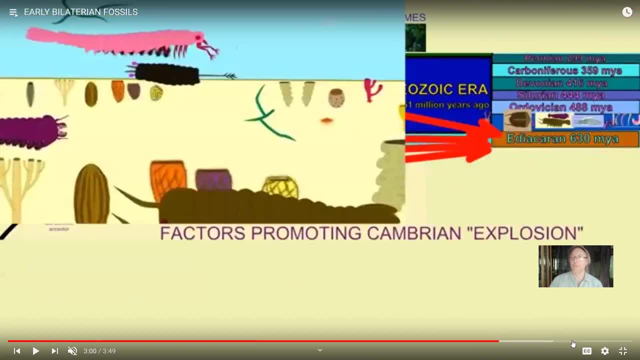 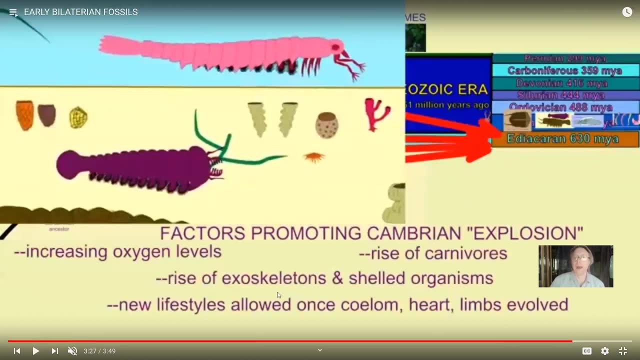 diverse branches of this family tree which then allowed for this Cambrian explosion, the great diversification of animals. Also, at the time of the Cambrian, oxygen levels had been steadily rising and were rising still. There were now carnivorous animals. so perhaps this would provide. 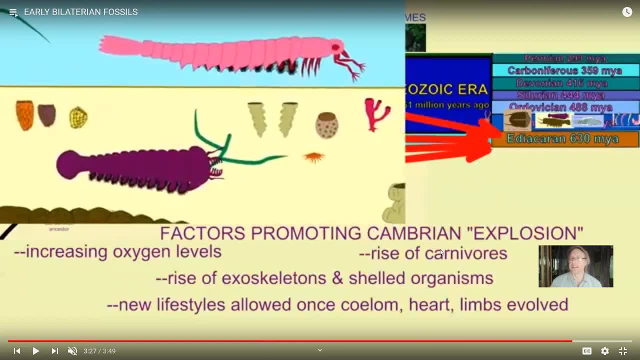 a selective advantage to more diversity in those organisms that wanted to avoid being prey. Exoskeletons were becoming more common, so arthropods, mollusks and others were providing protection for themselves, And then, once these animals got complex to the point that they did develop a heart or limbs or a 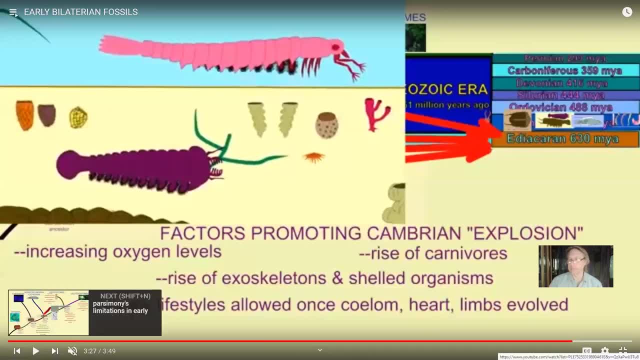 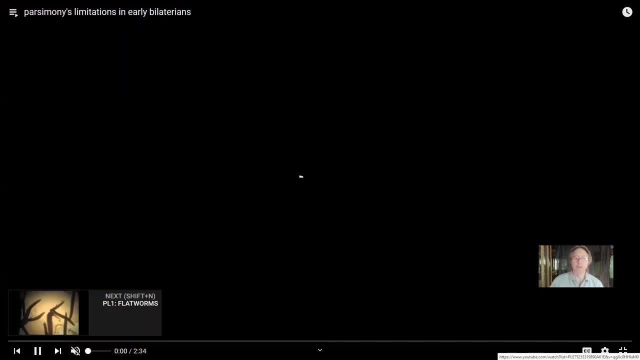 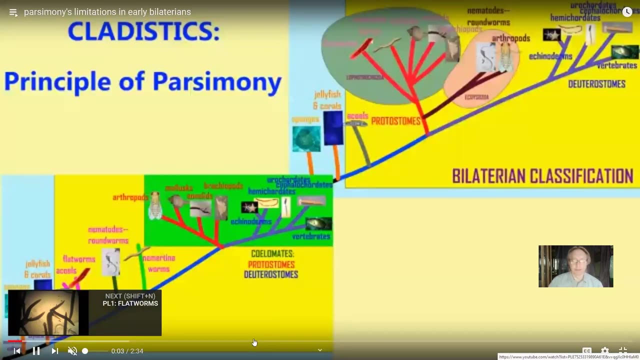 body cavity like a sea loam, then this would allow new possible lifestyles and then even more diversification, And so so far, so good. The problem then becomes- and you know, this is my personal perspective- is that if we don't develop a heart or limbs, then we don't develop a body. 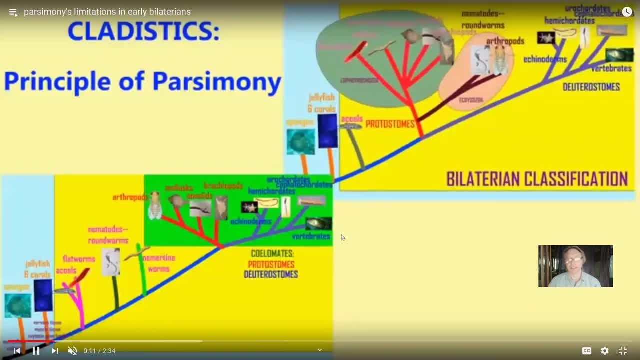 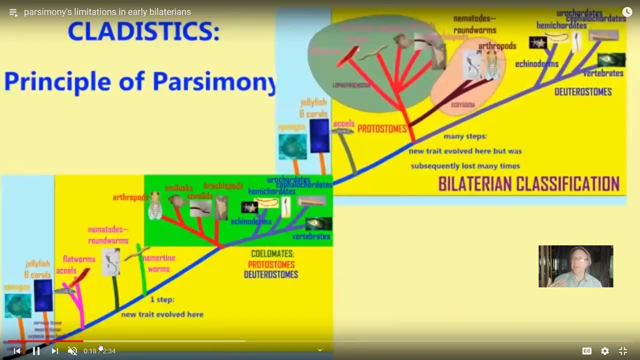 cavity. We reject the older classification system and accept the new one. The problem is that if you were to ask when did certain traits evolve, like segmentation or a heart or cartilage or limbs, In this model it's relatively simple And in the old form of classification a great emphasis was. 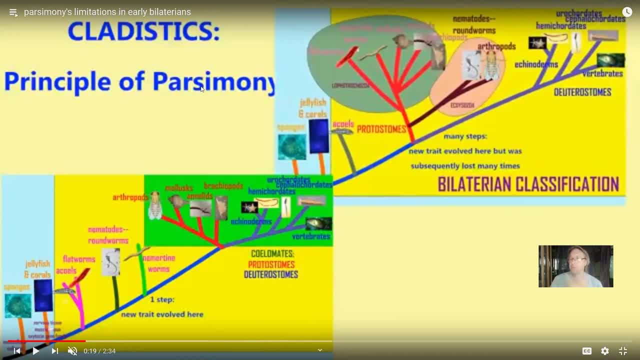 placed on parsimony, That means getting from point A to point B, getting from point A to point B and getting from point B to point B with the least number of steps. So if you're saying I think life evolved this way, that this evolved and then it went away, and then it came back, and then it went, 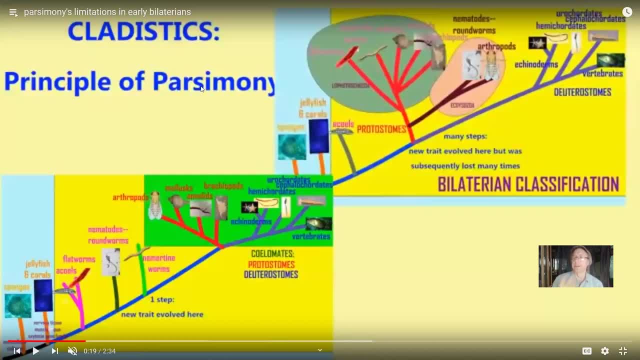 away or something like that. that's too complex, Just you know, proposing that you know, this evolved once and that all animals which have this have it from a common ancestor. that was, you know, preferred. It was more parsimonious, There were fewer steps, And so in this old model, if you 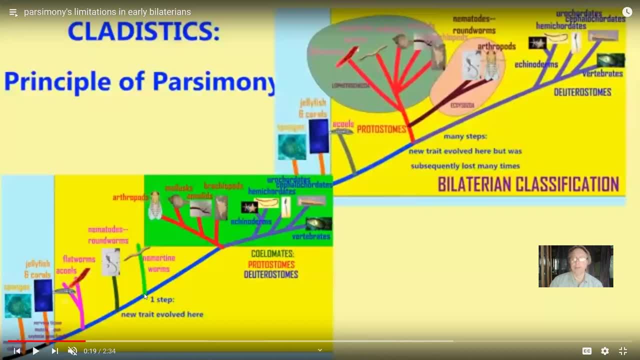 were to ask: where did blood vessels evolve? Well, they evolved here. And then everyone that has a blood vessel, you know, get it from this one point- And the animals which don't have blood vessels- they evolved in the family tree prior to that Segmentation- would evolve here, limbs would. 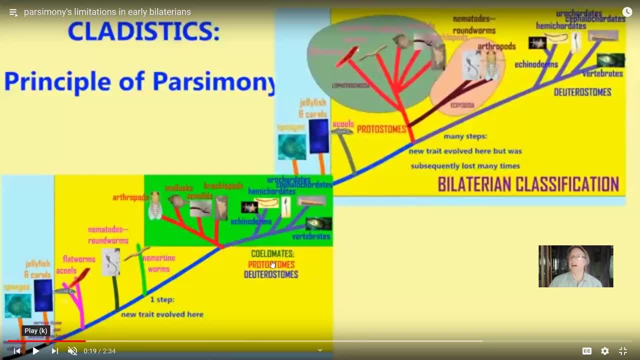 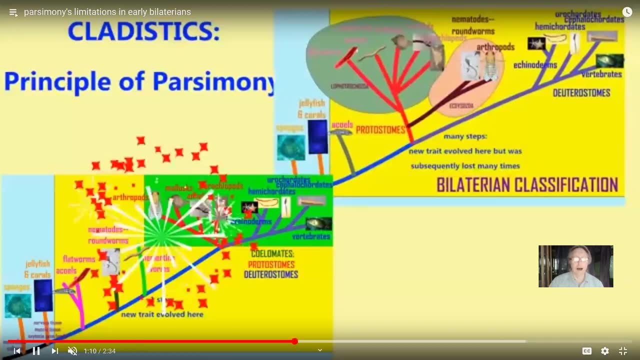 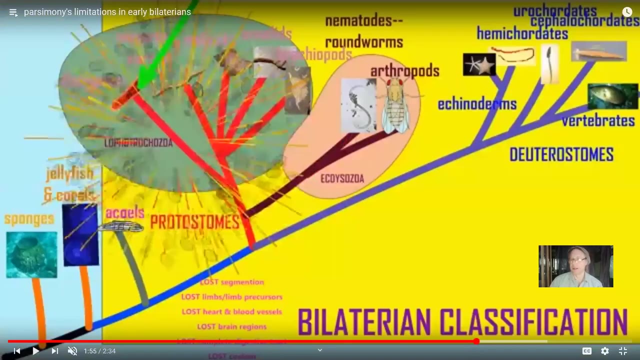 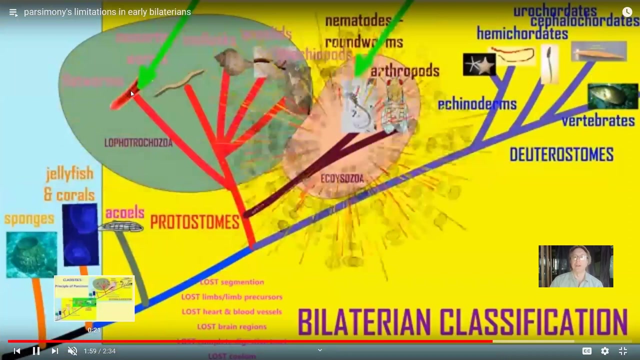 evolve here, etc. Now, in the revised classification, the genetics seems to support that. But the problem then is that it is no longer parsimonious when it comes to the parsimony, The traits, the anatomical traits. So, for example, here is a flatworm, now in the same group as the 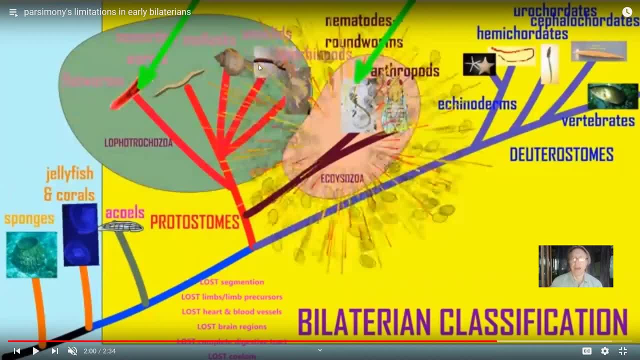 mollusks and the annelids. So the genetic comparisons seem to support that, But while these have segments and blood vessels and a body cavity, flatworms do not. While arthropods have segments and limbs, nematodes do not. And so then the question is: 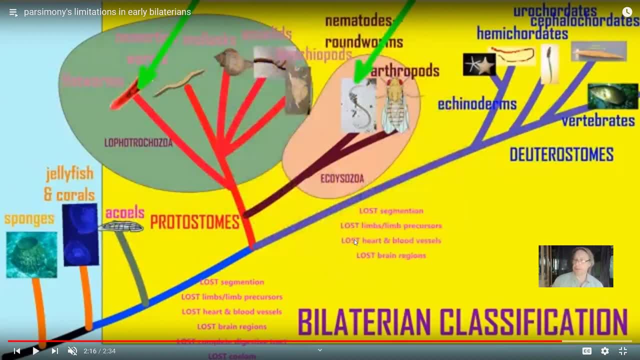 how did that happen? Did these traits evolve separately, Right and with some like a body cavity? you know, anatomically that does seem that it quite possibly evolved separately. But when we compare, say I don't know, say a vertebrate like ourselves and a fruit fly, when we tell our embryos put an eye. 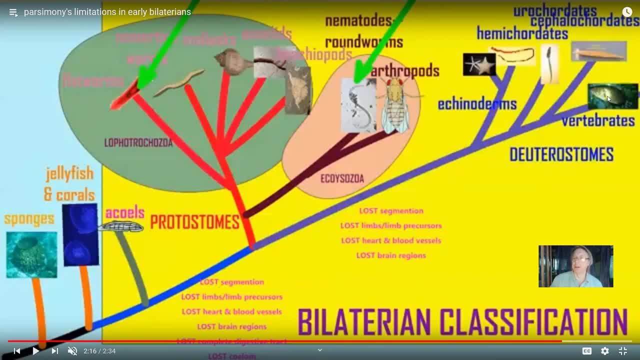 here, or put a heart here or put limbs here. we use the same genes. So this suggests that the genetic mechanisms for eye development, or heart development or limb development evolved once, which was shared by these things. that, by the point, you get here. 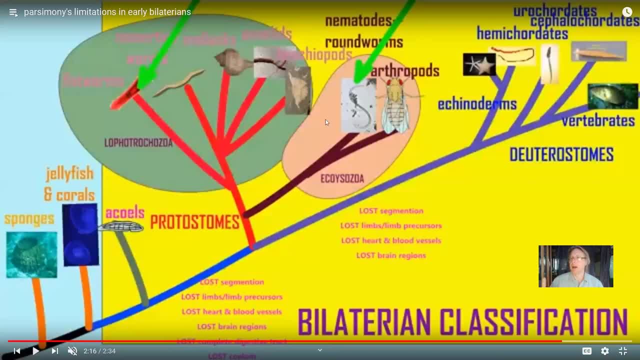 there were the features that their descendants would share. But then the problem is, these animals don't have those traits. did they lose them? These animals don't have these traits, did they lose them? And so then, in this model, it seems to suggest that a number of traits 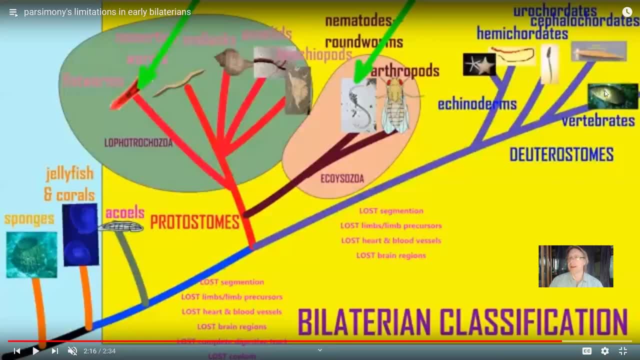 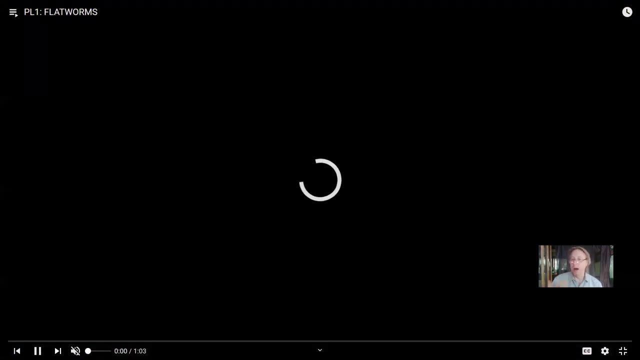 were present in this common ancestor, that these animals, these animals and these animals would share, but that some lineages lost them. And so, like I said, in science, I mean this is frustrating, but it's good. This is how science works. 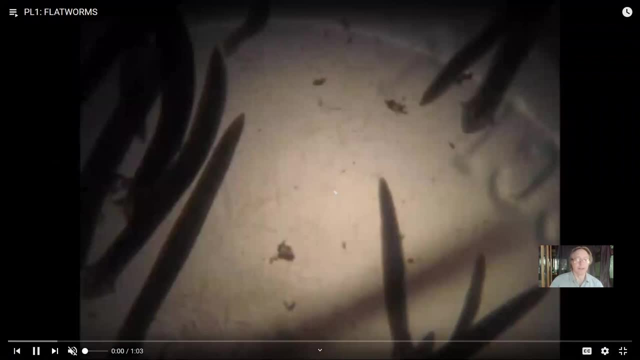 The answers aren't known. All that can then be said is: here's an idea, here's the evidence that supports it, And then later new studies- genetic analysis for example- could be proposed which say: well, let's review this. 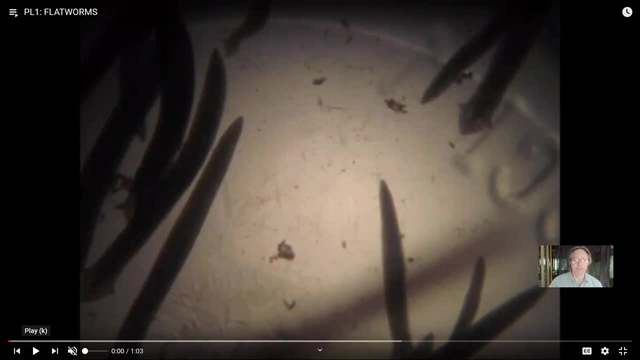 could we revisit that? Could we revise this? So that is the way that science is supposed to work, And nothing has ever felt that we understand this 100%. anything could be changed. We used to think this, but now we think this. 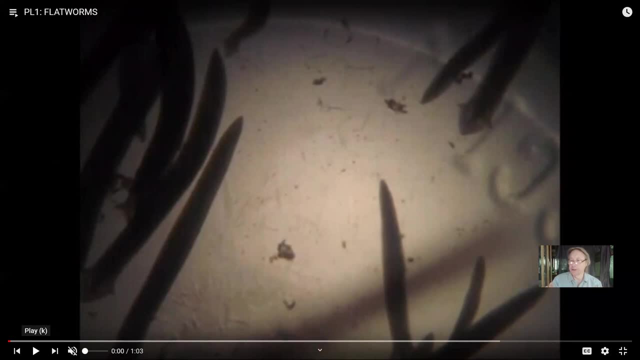 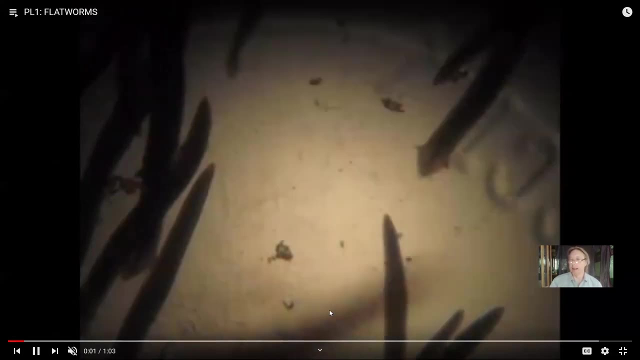 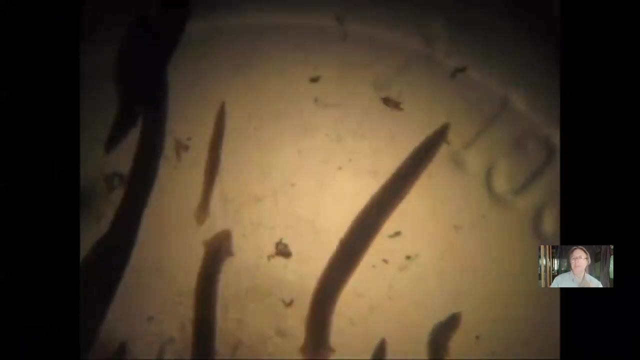 So scientists are still debating the relationships and the branching points and the different points of the animal family tree. So these flatworms, they are bilaterally symmetrical and thus more advanced than than jellyfish, but they certainly lack many of the features. 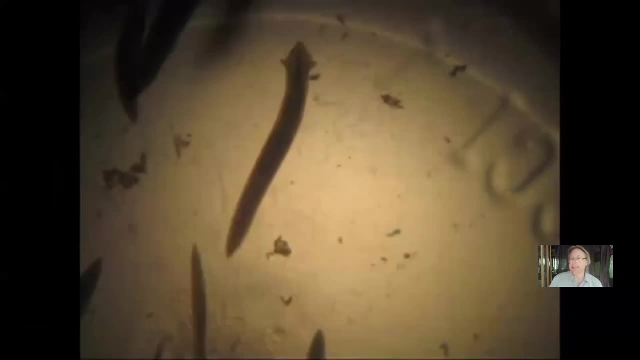 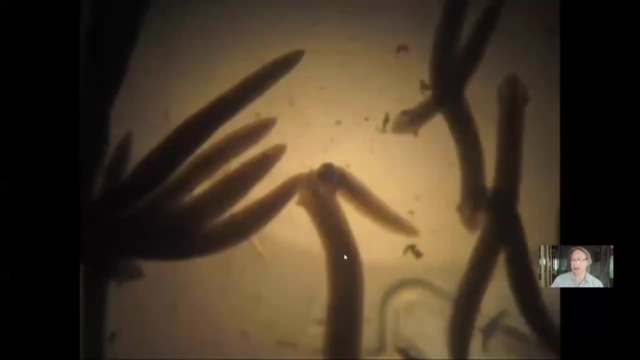 which would come later. For example, these still have a centrally located mouth, So planarian have a mouth in the middle of their body and only one opening. So it is a incomplete digestive tract And once again there seems to be a difference. 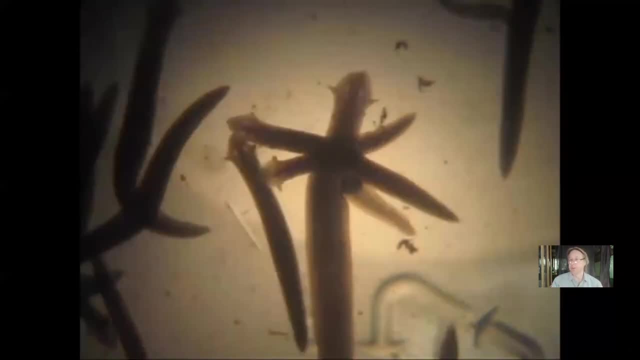 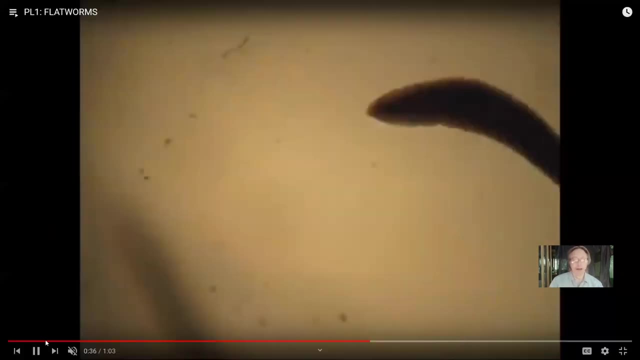 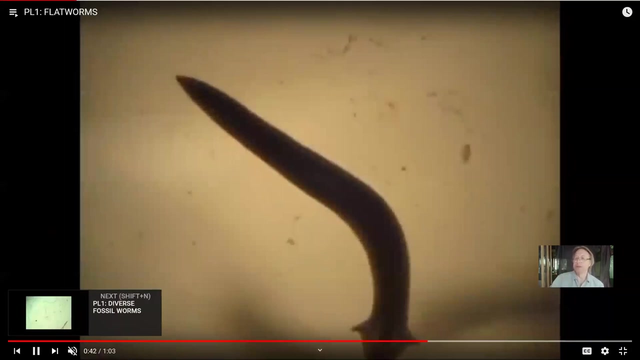 in biologists, cladistically, using parsimony, that would make these primitive animals but genes, you know, would then suggest an alternate form of branching. Now I would like to move past worms, but just a quick thing that most people don't know. 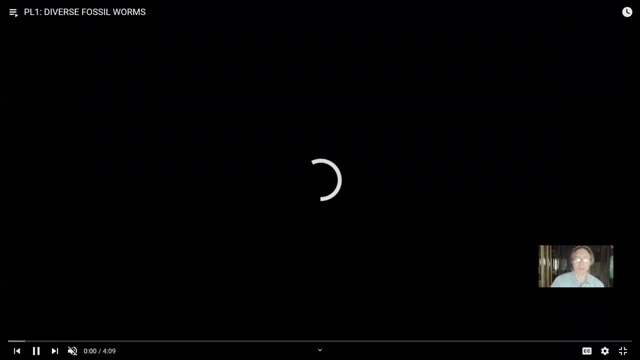 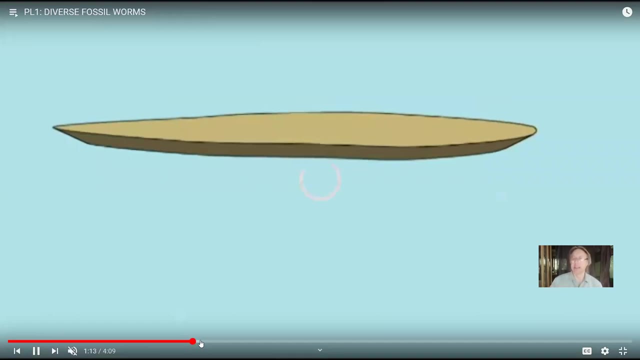 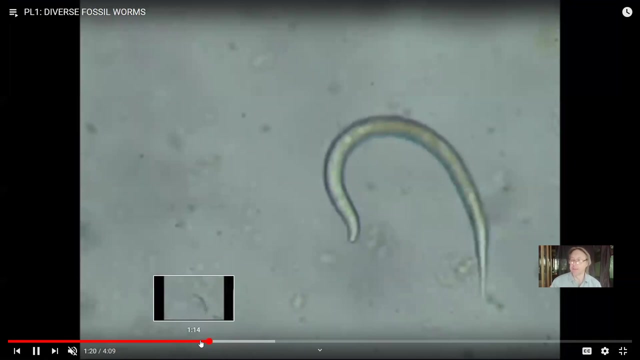 There's lots and lots of different kinds of worms, Some of which are microscopic, including what is at least the second most successful group of animals on the planet in terms of species. So arthropods seem to be the most successful. But these worms, these nematode worms, 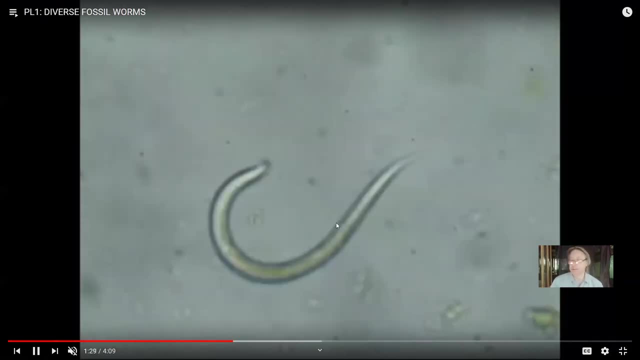 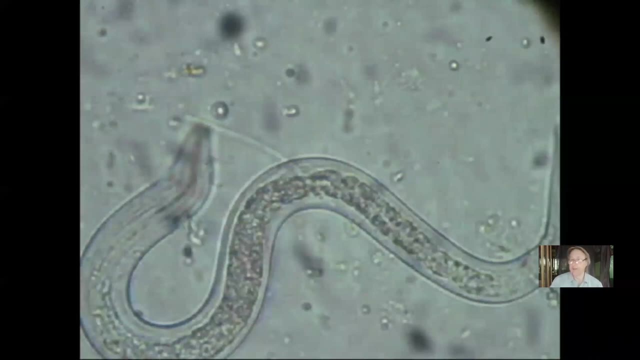 which are unsegmented round worms. these, in terms of number of species, are the second most common. Whenever you walk on soil, you're walking on them. They're everywhere, And while some are intestinal parasites and some can be visible to the naked eye, 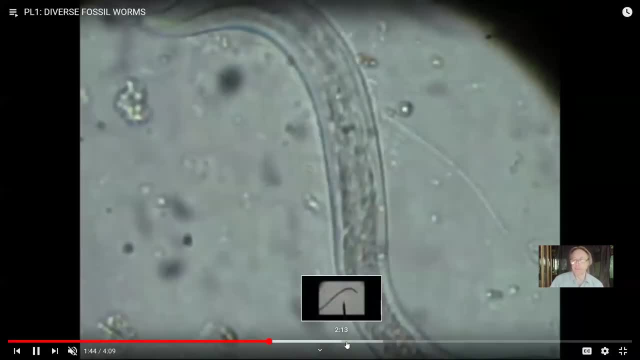 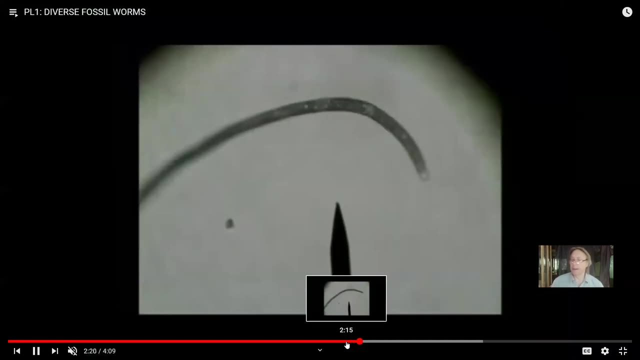 the majority of them are microscopic, And the reason I'd like to stress this just for a little bit is that when we think of animals, we often think of the big ones. Even when we think of worms, we can think of the big earthworms. 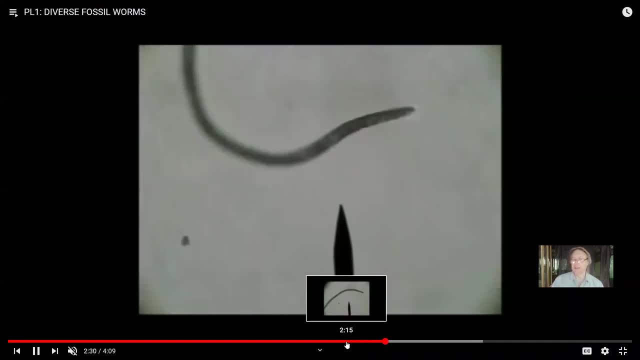 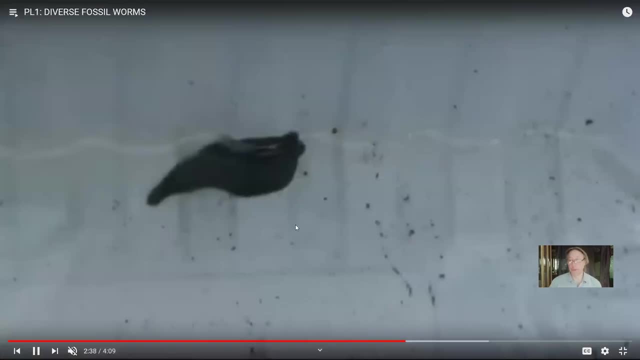 But the reality is that many animals- and actually given just the huge number of you know nematodes, arguably you know a huge percentage, maybe even most animals. nematodes are more common than we think they are. They are microscopic. 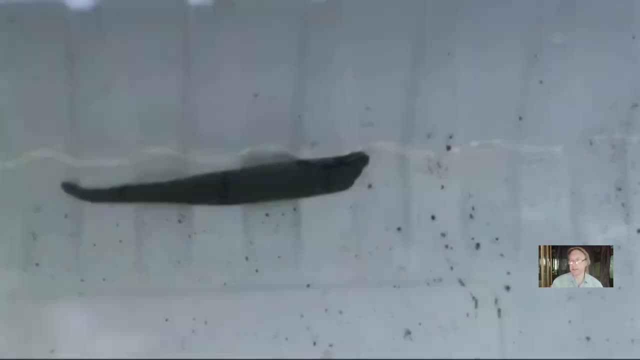 So what does that mean? It means that when hearts first and second first developed, or blood vessels first developed, or respiratory structures, if you're thinking of, oh, how does this big animal evolve a heart, or evolve a brain? 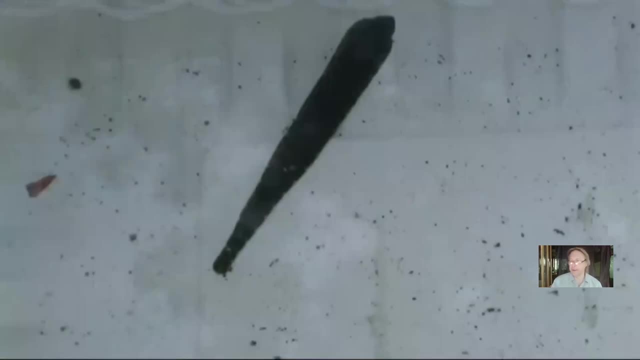 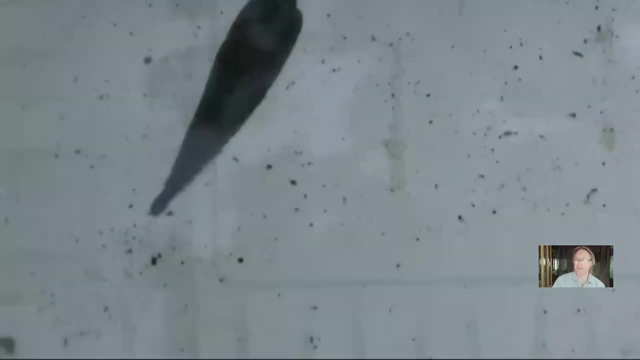 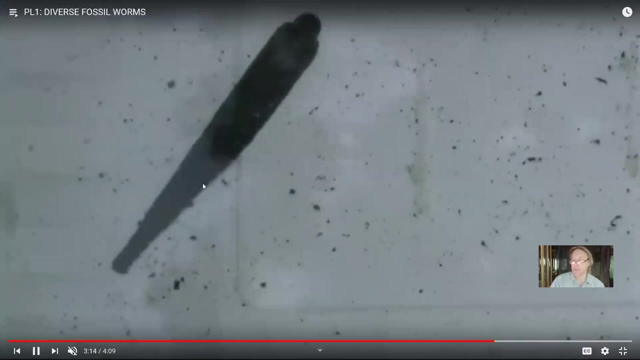 But when you're dealing with microscopic animals, well, really, you know, these most primitive structures would have been rather small and rather simple. So many of the advances of animal evolution occurred in much smaller animals. Now here's a segmented worm. It's like an earthworm. 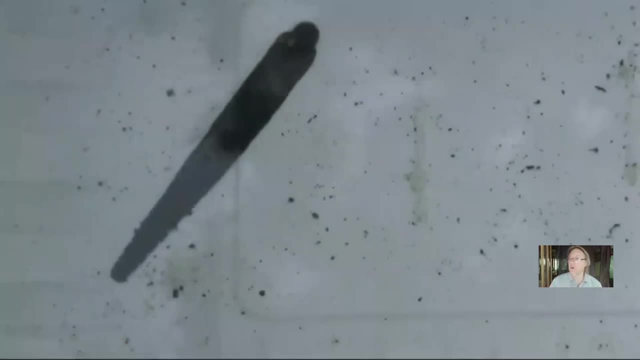 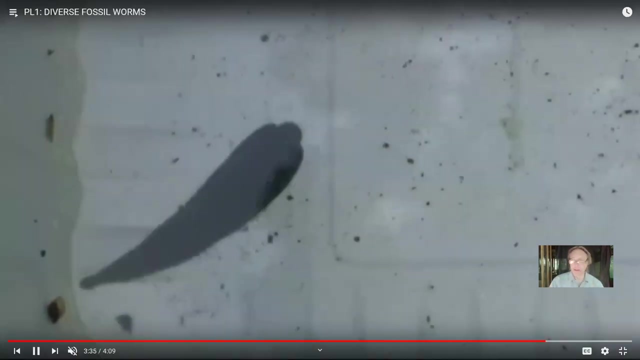 So this is a leech. It's like an earthworm. They are far more complex than nematodes. In addition to being larger, they have a body cavity, a coelom. They have a heart and blood vessels. They have more layers of muscle. 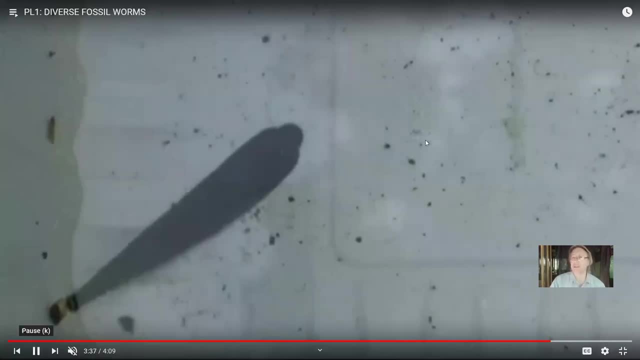 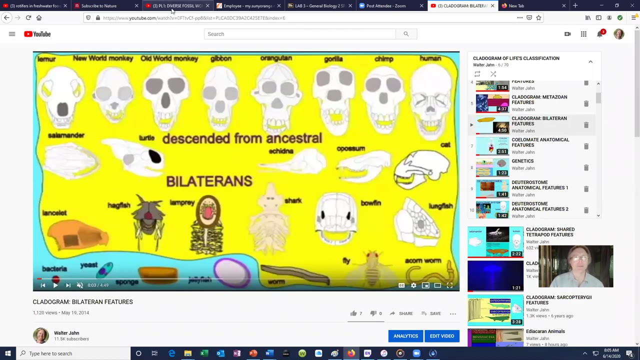 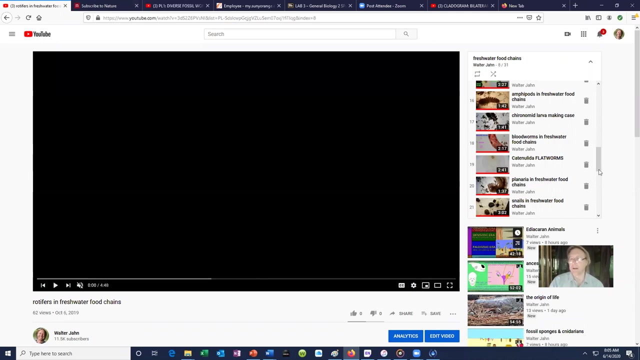 They in some actually then even have limb precursors. And so there are all of these different kinds, you know different kinds of worms. Now there are a few more worms. I just you know. once again, I would like to point this out. 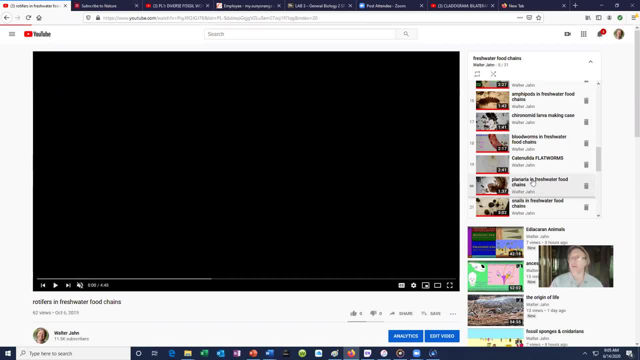 that when we talk about worms, like even in a pond near yourself, there's all of these different kinds, And so, as I zip through invertebrate fossils, then we're just not giving a comprehensive view of the groups of invertebrates. 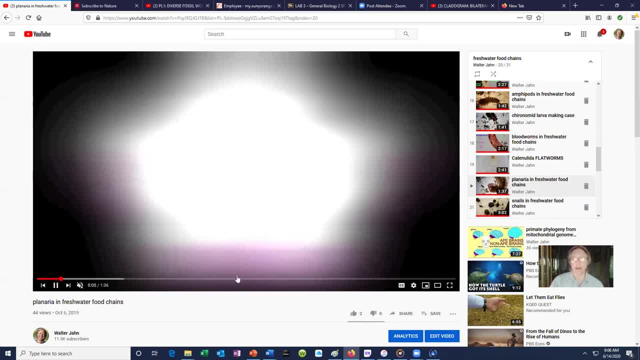 There are just far too many. So if you were in a pond, you know, in a pond, you know, if you were in a pond near yourself, you would certainly, you know, be able to say, find flatworms right. 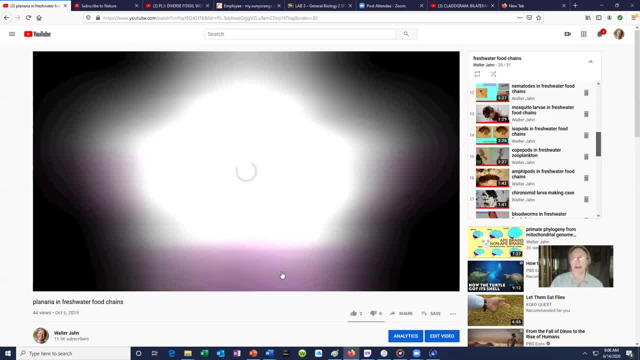 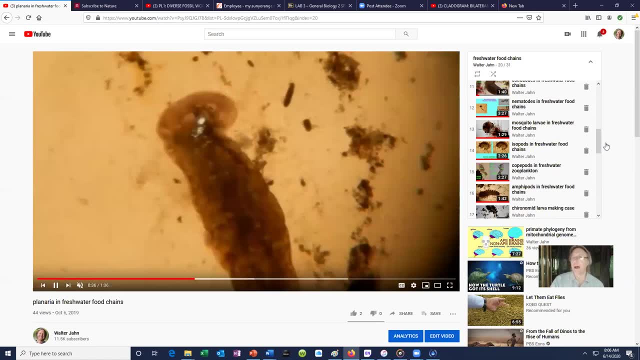 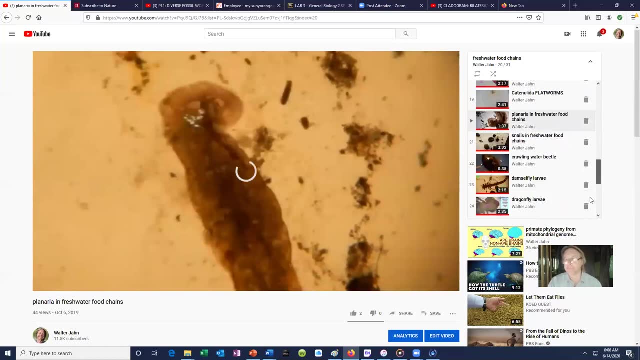 Well, that's when you've already seen some. you just jump ahead. So you know, here's a flatworm, the planaria that you originally saw. they were pretty big, but there are certainly smaller ones as well. We are used to, I'm sorry. 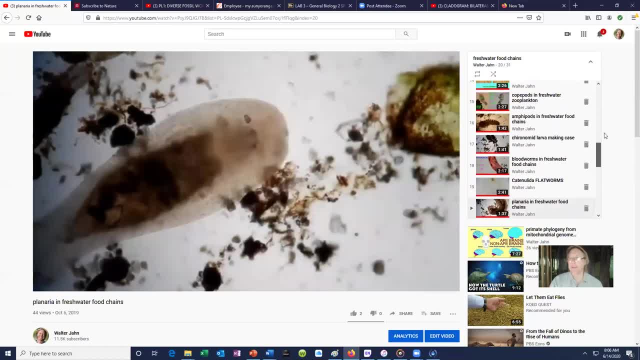 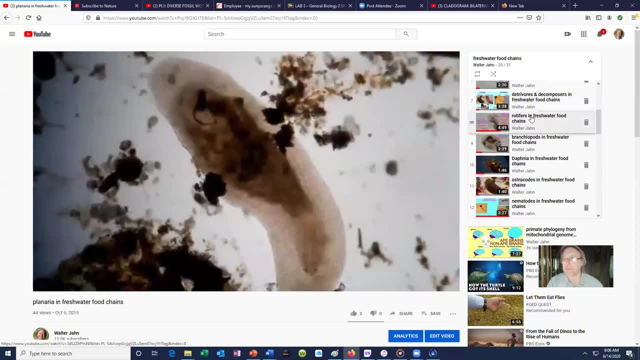 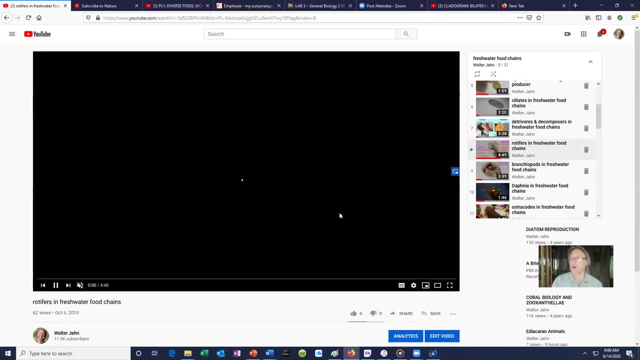 we are used to earthworms- I'm being large but there are many smaller animals. I'm sorry, I'll get to worms in a second. There are other bilaterally symmetrical animals which are simple, which aren't worms. 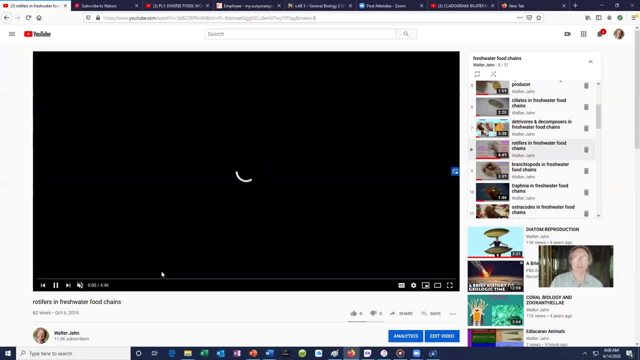 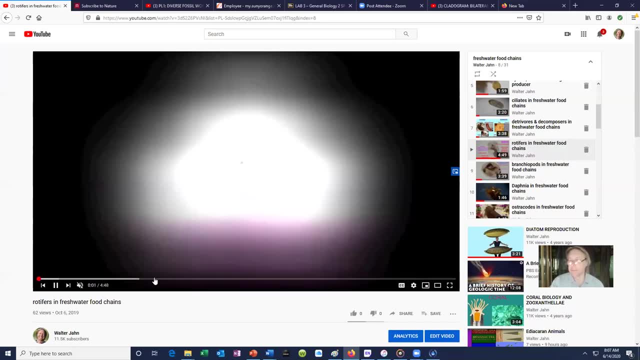 So, example: there's a group which are microscopic, or nearly, so called rotifers. They are very common. So this is a microscopic animal but nevertheless it has a complete digestive system, It has a brain. So even though it's microscopic, 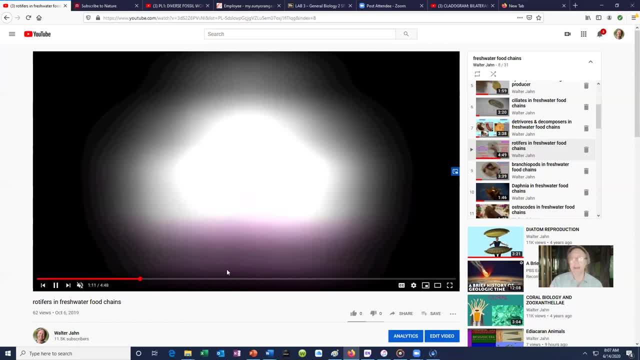 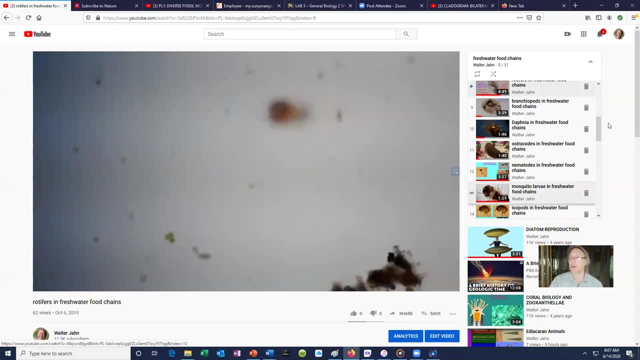 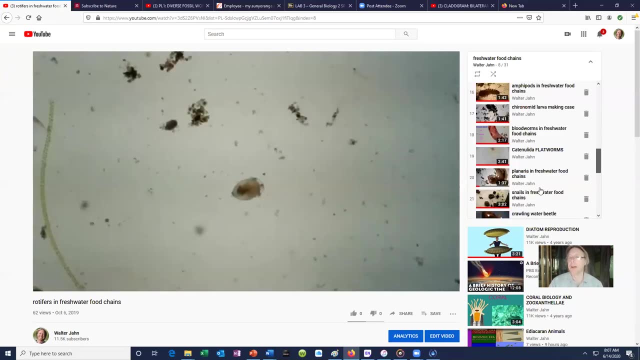 it is complicated, even though there are one-celled paramecia which are larger than it, And so there are actually animals which are smaller than one-celled organisms. Once again, as we talk about, how could animals possibly have, you know, evolved? 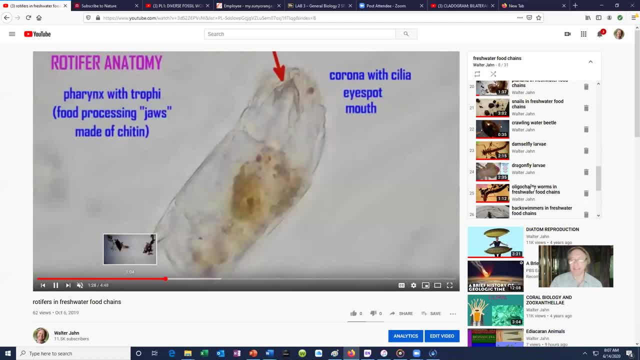 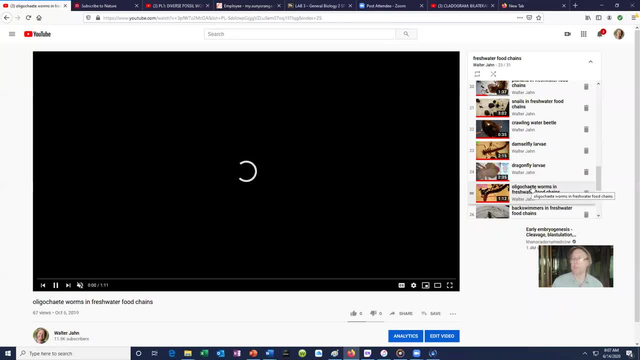 When we think about leeches and earthworms. they're big, they're more complex, but they have cousins which are microscopic segmented worms. So once again, I just wanted to introduce that point that a lot of people don't think of. 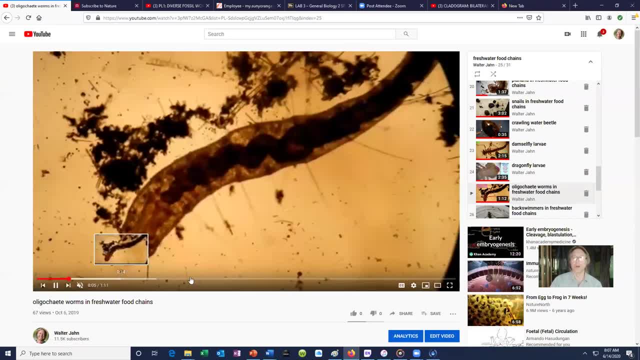 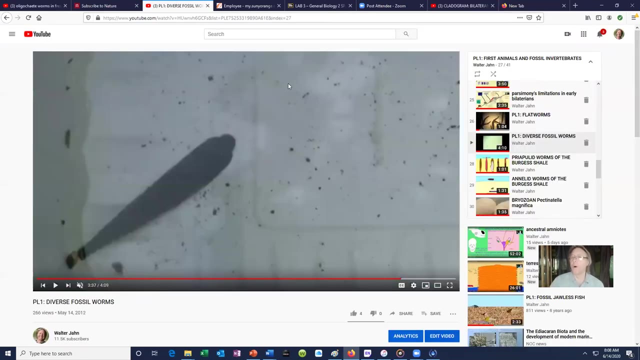 First off, there's lots of kinds of worms which aren't closely related to each other at all, And many animals are microscopic. And so when we're talking about talking about the evolution of groups, especially since so much of this happened in the in the Ediacaran period, All we have are worm, you know fossils, So we know they were worms. 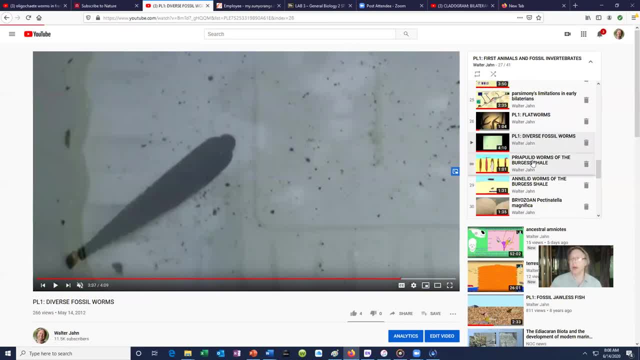 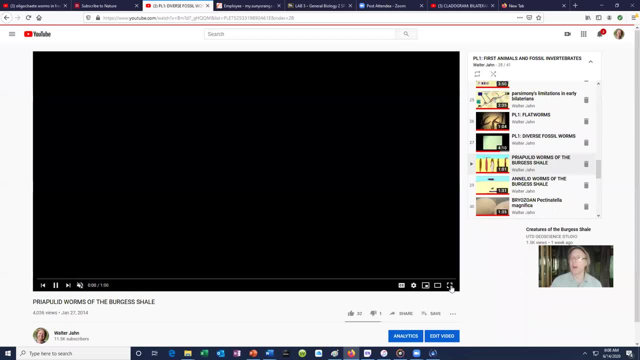 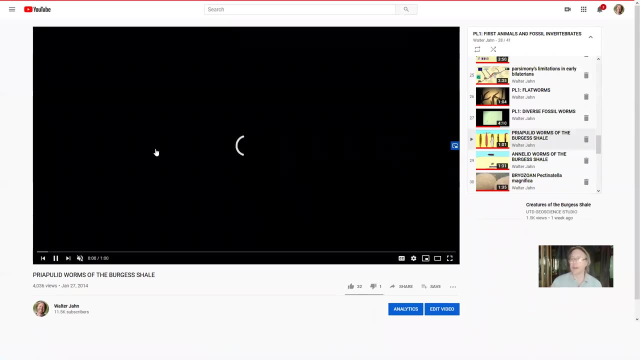 if we like, see fossils of a burrow, for example. But which of the many kinds of worms? that's a question. By the time the Cambrian comes around, some of the dominant predators are worms. These are still alive today, although they're not very common. They're called Priapulid worms. 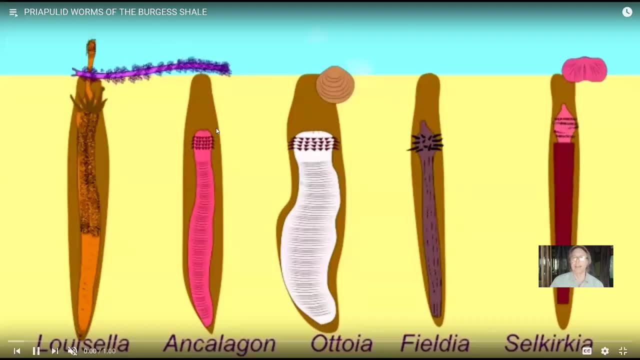 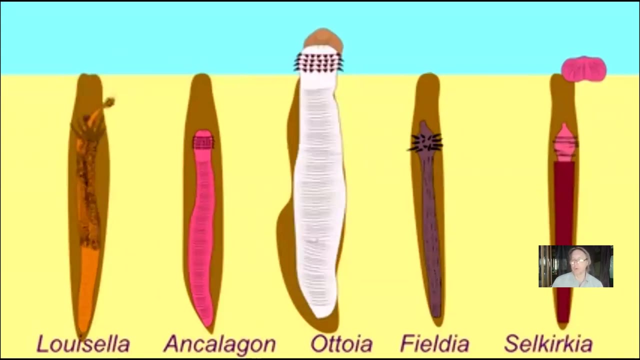 So these were large worms which would perhaps sit in burrows and then come out and ambush their prey. Once again, these were dominant predators in the Cambrian, capable of even feeding on shelled uh organisms. And so, um, once again, you know as the Bilaterians diversified. 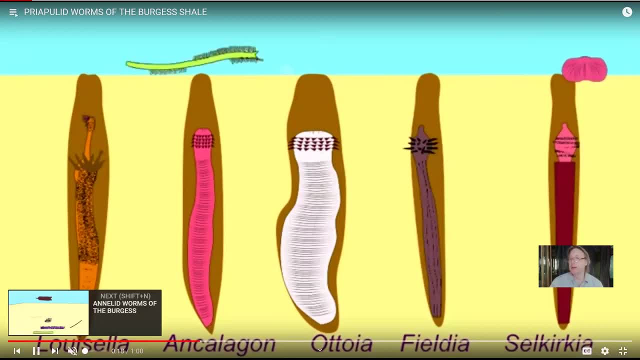 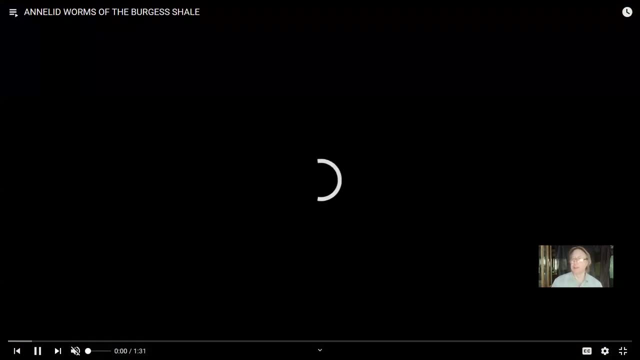 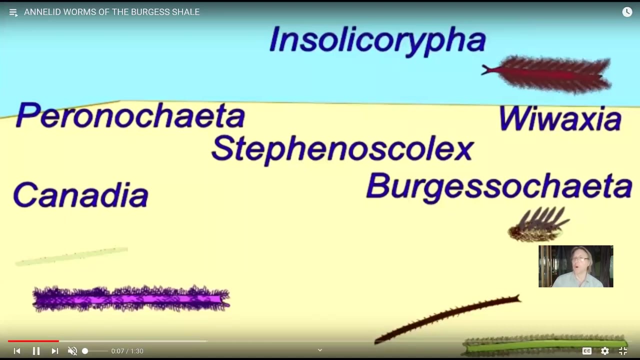 this included a great diversity of worms. Claudina, which lived at the end of the Ediacaran period, had a shell around itself, So there were even, you know, shelled uh worms. Um, some of the worms, uh, that exist by the Cambrian are segmented, So we certainly know that, um, you. 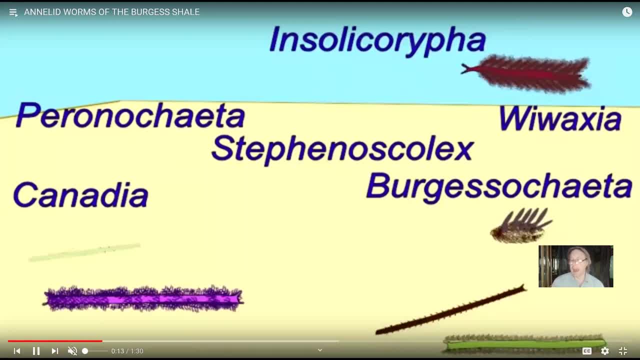 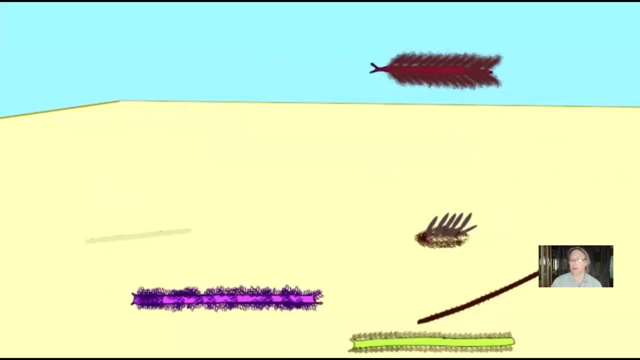 know the Anilids, which today would include leeches and um and earthworms, but also other forms, like the microscopic one that I had just shown you. Even though worms technically don't have legs, many of them do have lateral outgrowths which can serve as a respiratory structure. 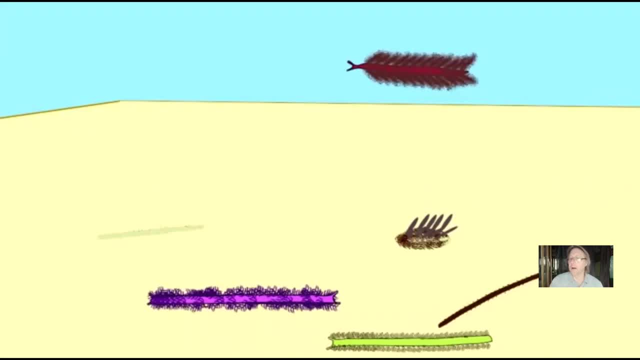 help in swimming or even help to move them along. Um and so, even though they're not technically legs, nevertheless worms can have a series of- you know- structures involved in locomotion, And some of the genes they use to make those structures are homologous to the genes that say: 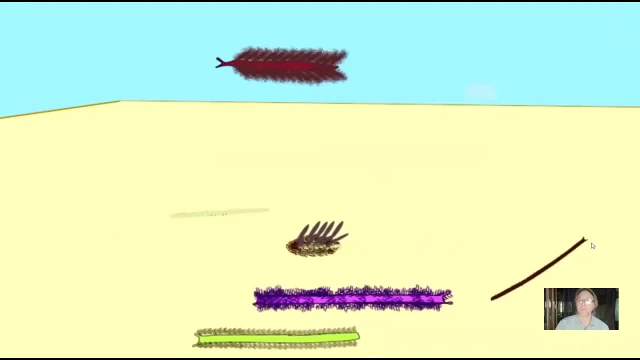 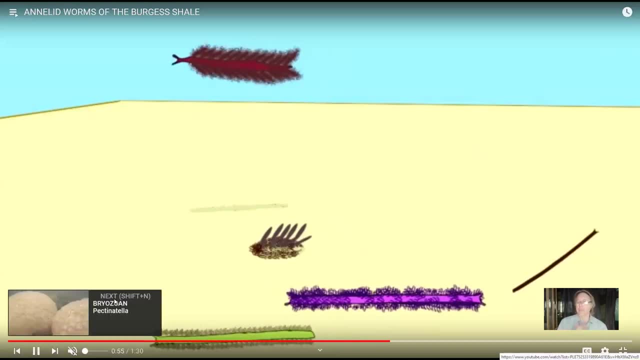 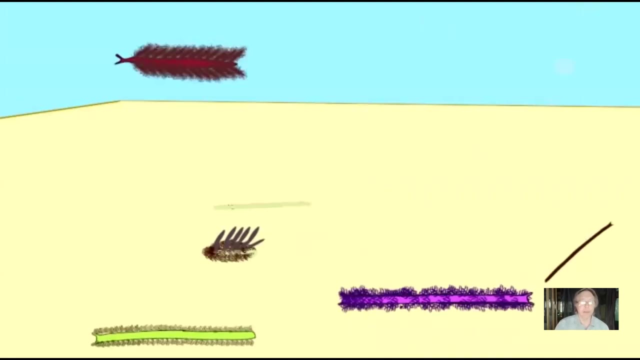 arthropods or even vertebrates use for their limbs One uh worm. uh was known to be uh armored, And so um worms evolved in the Ediacaran period. They were coming becoming more complex. by the end of the Ediacaran period And then by the um Cambrian period, there was a 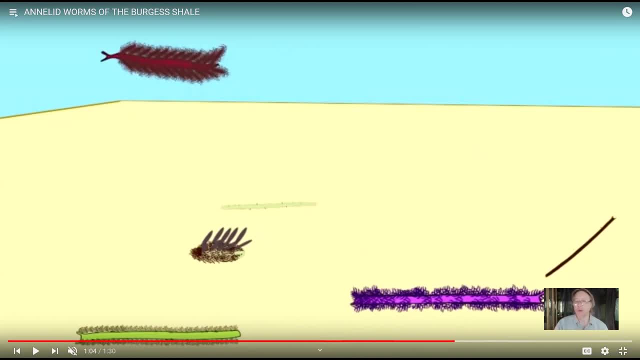 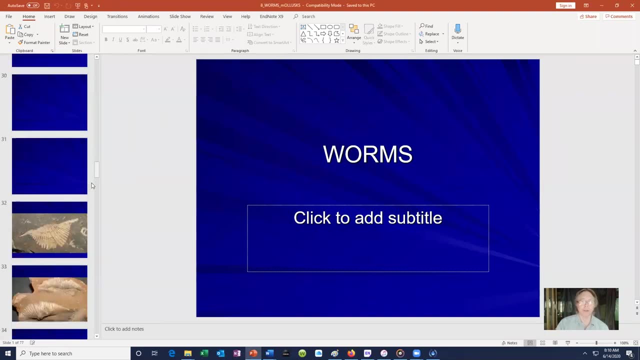 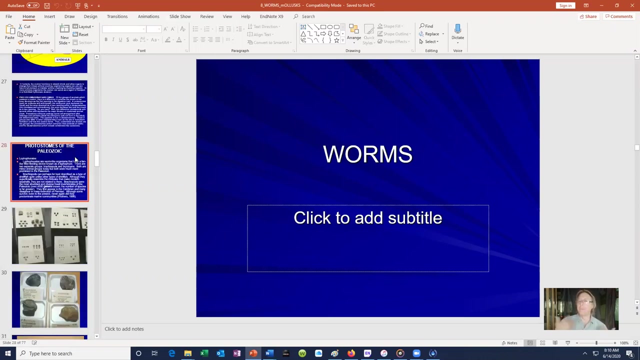 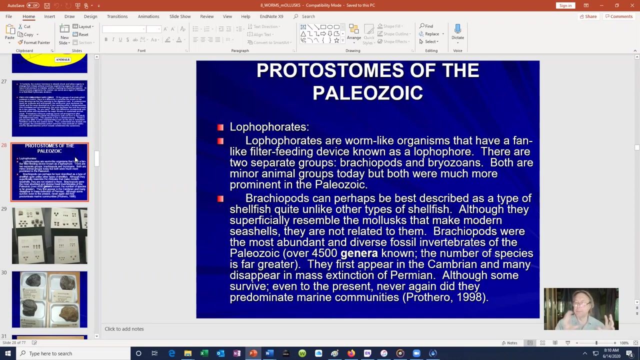 great diversity of worms, Um, which aren't closely related to each other. Um, and today there are a great diversity of worms, uh, known, um, which are not that closely related to each other. Um, some of these worms had body cavities and uh, of the ones which had body cavities, we lump, you know, uh, you know. 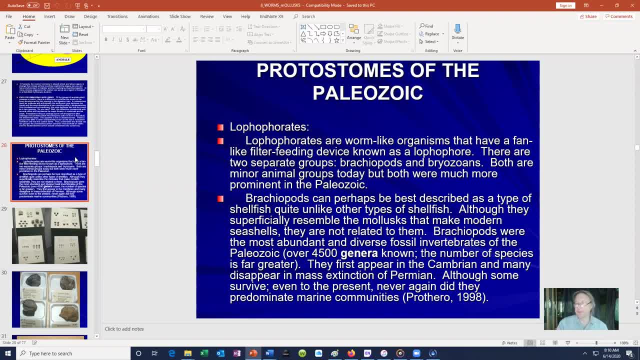 many in the protostomes Uh, and one of the features is that uh, when they develop as their mouth develops from the first embryonic pore and the deuterostomes uh, where the mouth develops from the second embryonic uh pore. So the protostomes include two big groups which 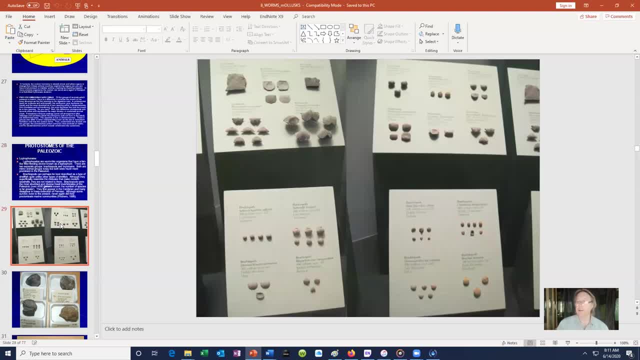 will get some focus: the mollusks and the arthropods, but they include lots of things that you've just seen: Some of the worms um, uh, the uh, the rotifers, um, but also then uh. 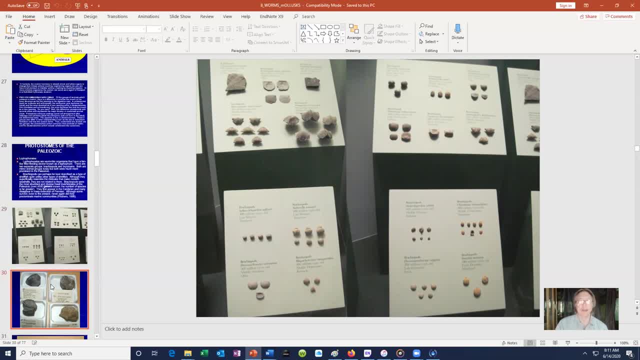 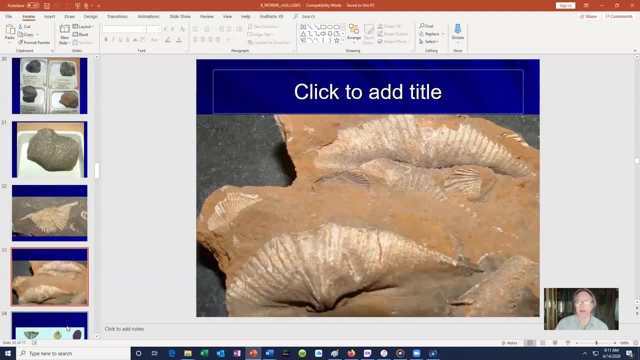 two groups called brachiopods and bryozoans. Now, these kind of look like clams, They look like mollusks, you know, they look like like muscles or scallops et cetera, but they're not, They're brachiopods, Although brachiopods are still alive. 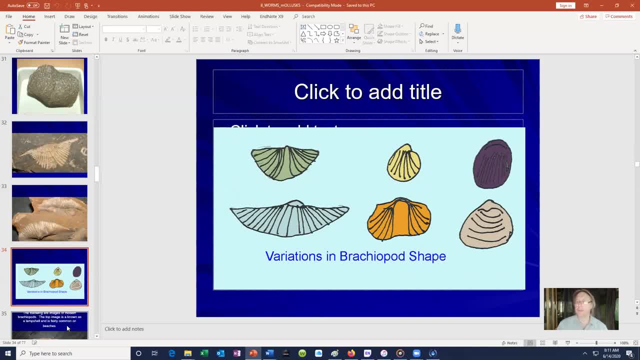 uh today. uh, they were far more diverse. in the Paleozoic These were the first dominant shellfish in uh the ocean. It would be at the end of the Paleozoic there was a mass extinction that really uh, limited uh. 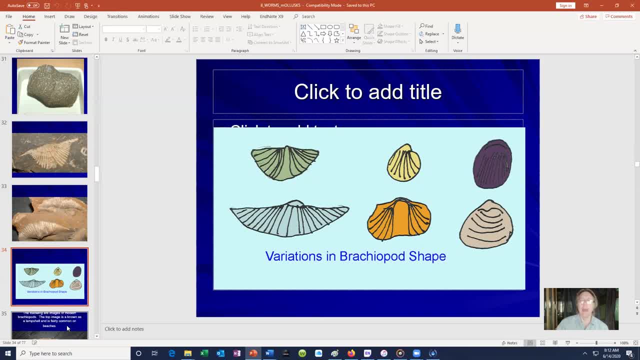 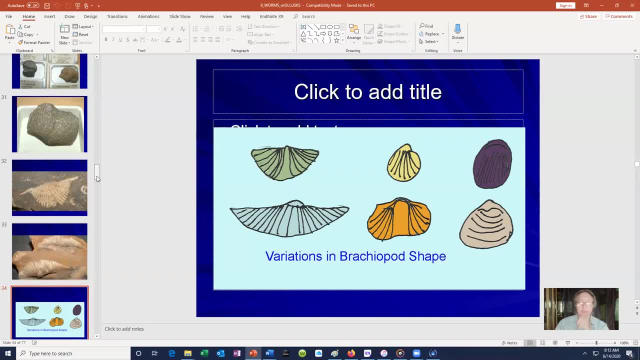 the diversity of brachiopods and that the um uh, the mollusks, uh, you know, with bivalves, like clams, uh, et cetera, they would kind of um really thrive afterwards, Brachiopods. 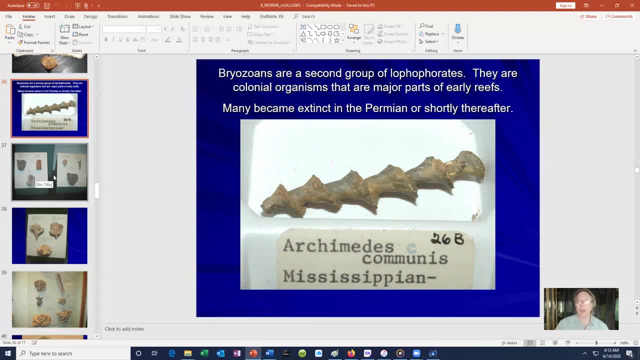 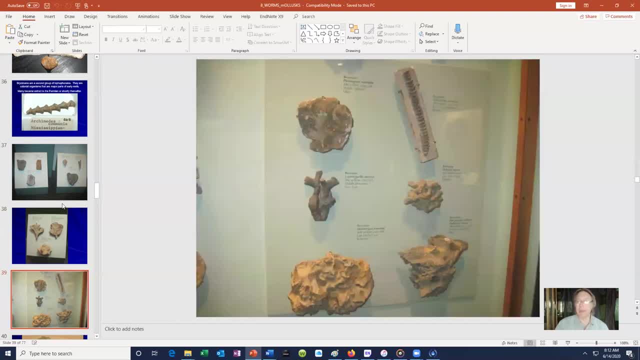 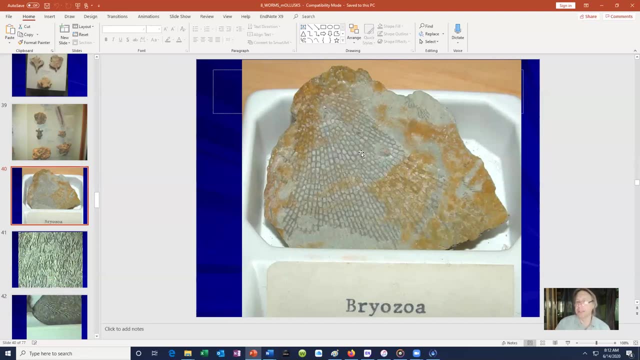 were related to another group called bryozoans, which once again had a very rich fossil uh record. And so when we look at the Paleozoic, so a bryozoan would include colonial forms, kind of like a coral. Each one of these little cells had a little 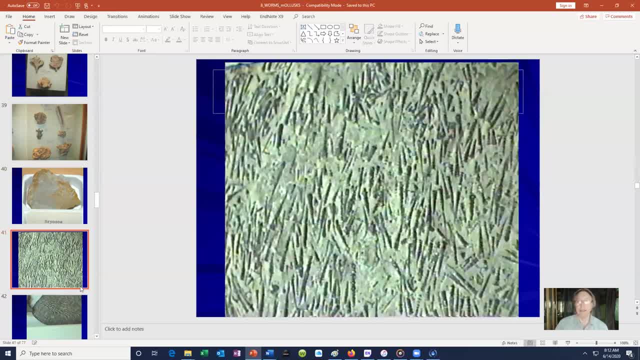 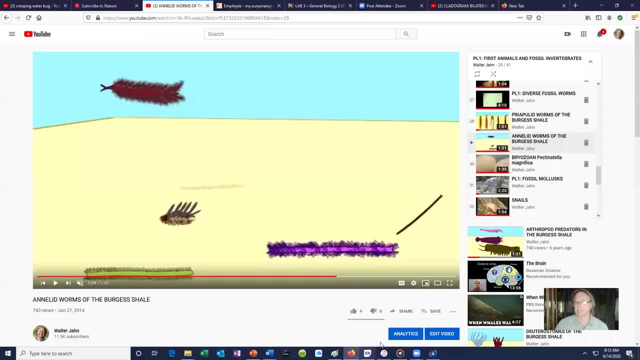 tiny animal and they kind of form a? uh colony And, as you can see here, bryozoans uh- bryozoans like Archimedes uh- were quite um uh common. Now there are still brachiopods which look like. 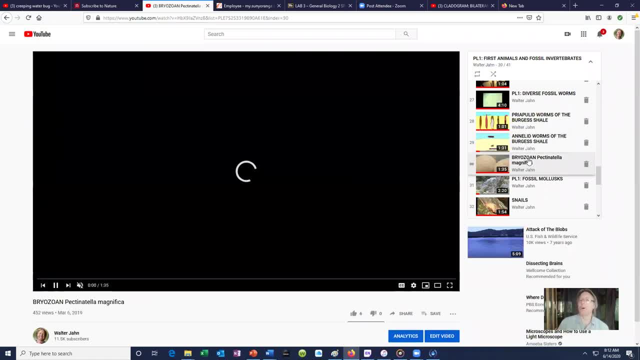 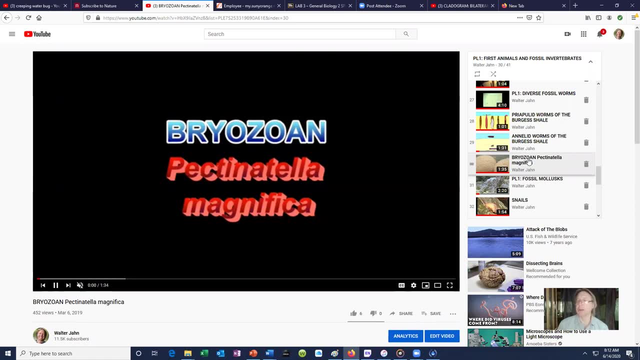 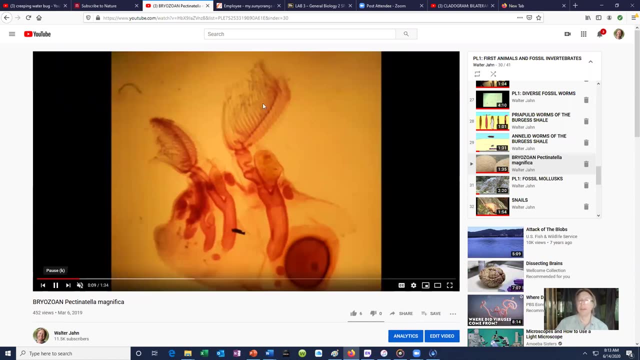 you know shellfish, but they're not mollusks at all. And there are still bryozoans alive uh today. So here's a bryozoan which lives uh in uh fresh water. Uh, so, um, both bryozoans and brachiopods, uh, they have uh a uh. 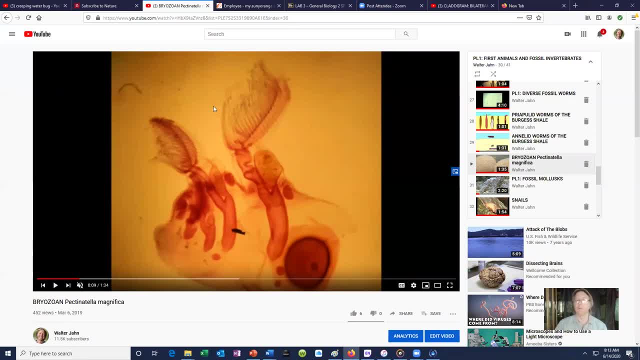 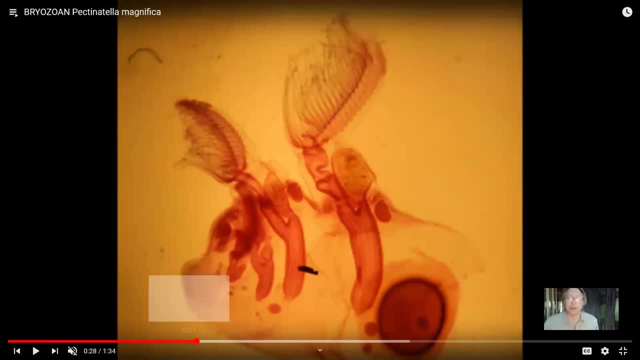 structure which they use to filter food, known as a lofophore. That's what that is, Uh, and so, therefore, they are classified um, uh, together in the same group, based on this shared anatomical feature. And um, if you were to visit, you know freshwater areas, um, you might. 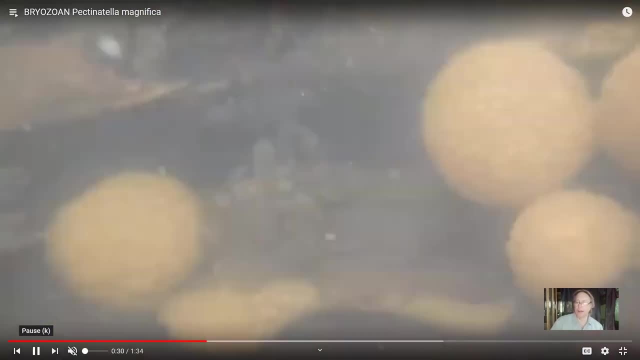 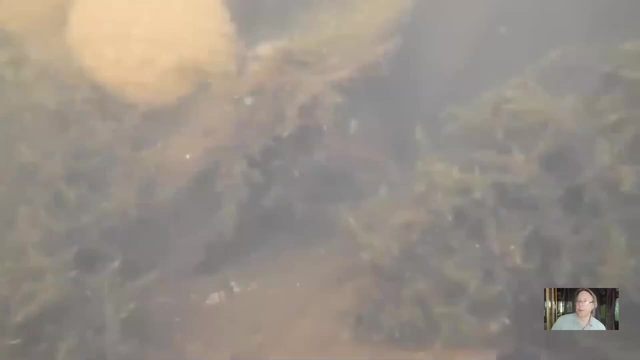 you know, find you know, this colony of uh bryozoans. So, um, I simply mentioned these because there's a great diversity of invertebrates, Uh, and so this course could never no, no one. 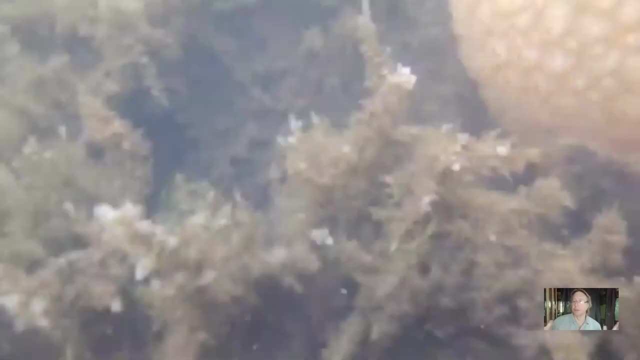 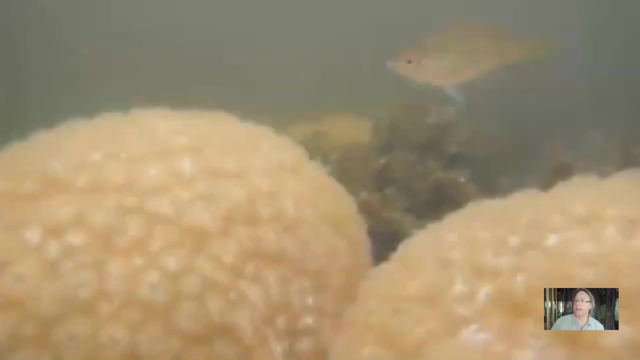 could ever, you know, uh, give a, you know, a justifiable uh survey of them, because invertebrates are so diverse And so, therefore, many of the fossil invertebrates you know, once again we are going to gloss over as as we go into the 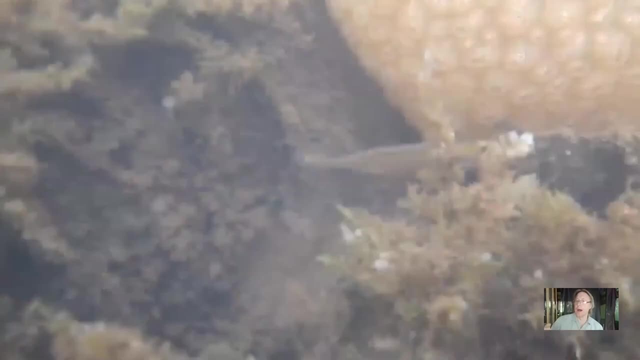 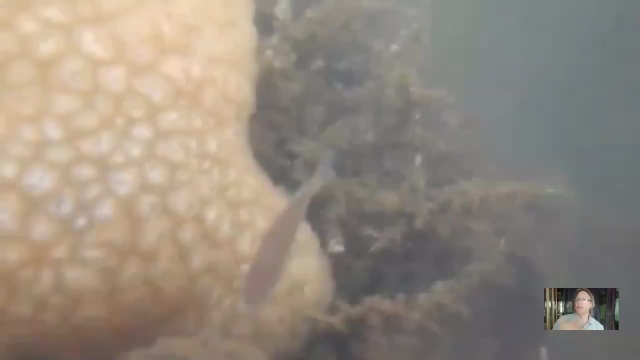 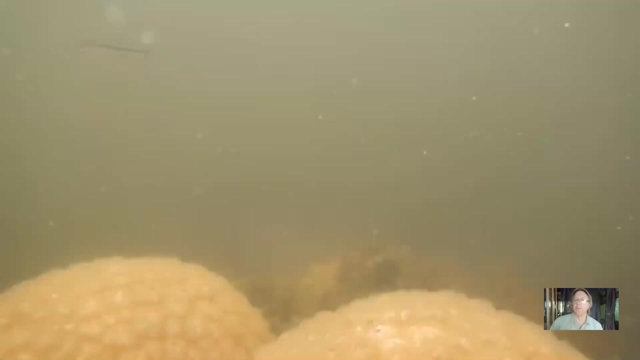 um, uh, the vertebrates. However, um, the Paleozoic is called the Paleozoic. It means old life, because if you were to say, go scuba diving in the Paleozoic, life would be very different. You would be struck by how different that life was from modern organisms. So for 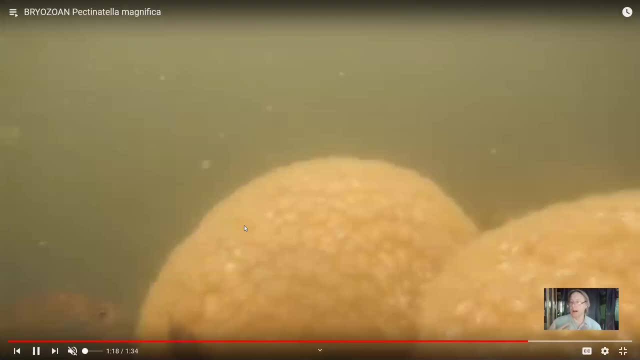 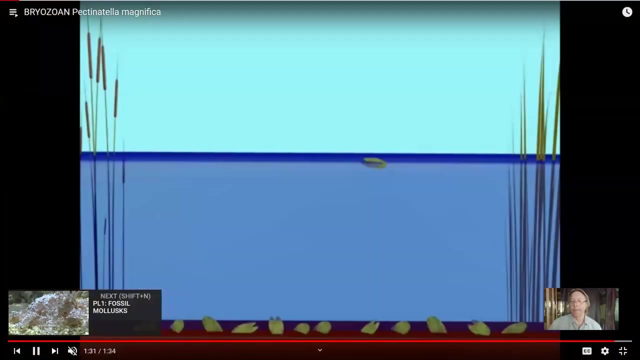 example, bryozoans and brachiopods, would be um predominant invertebrates, While today they are uh alive, they are minor uh uh components, Um, and so I simply wanted to to mention these when we discuss the uh uh, the mass. 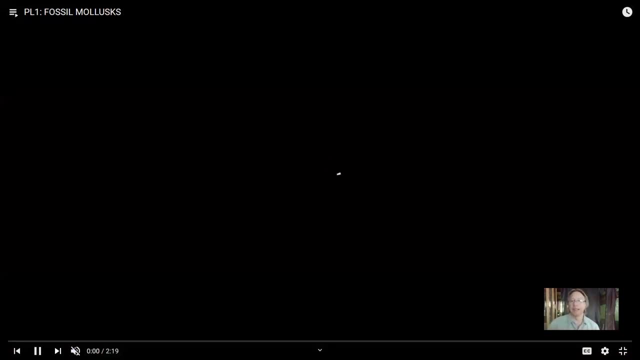 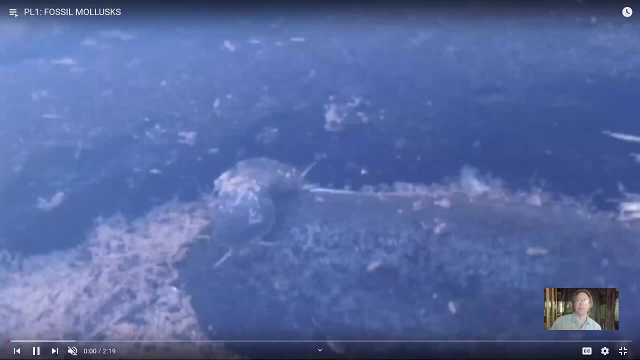 extinctions um. the mass extinctions in the Paleozoic, such as the end Devonian and the end uh Permian extinctions uh. many of these invertebrate uh groups have become extinct Um. the last group in this video I'd like to mention, um, is very successful. 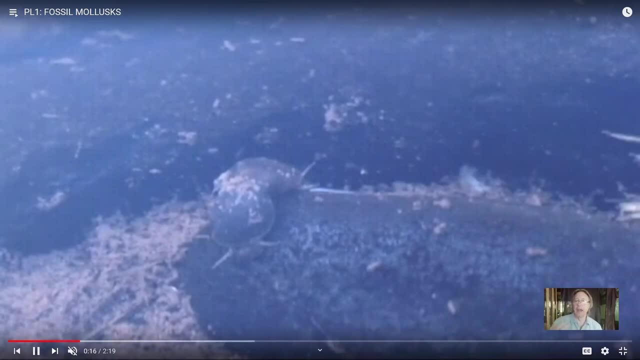 in the fossil record and is very successful still today. Uh, so these are protostomes. uh, so they are not in the vertebrate. you know part of, uh, the Bilaterian family tree? Uh, when they develop as embryos, their mouth comes. 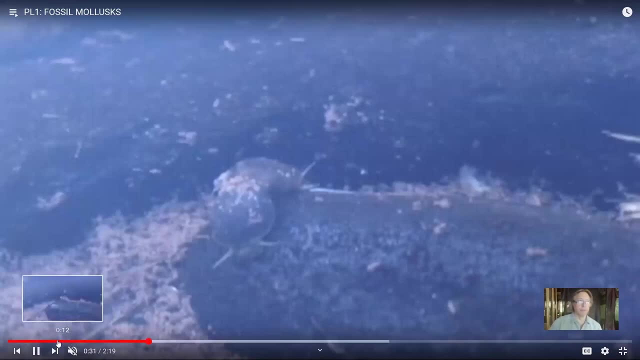 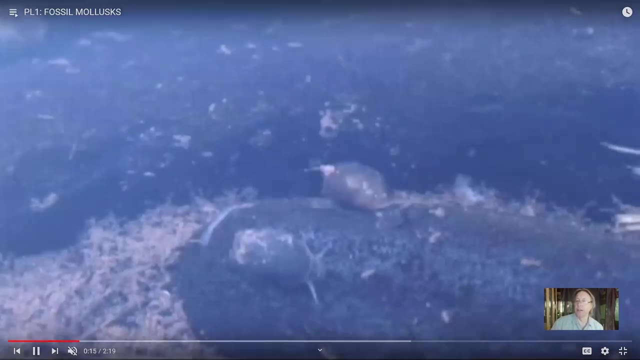 first, and there's a bunch of other features uh that make them different from the vertebrates and molluscs today, include things like uh snails, Like you see here, uh slugs, um uh the bivalves uh, such as. 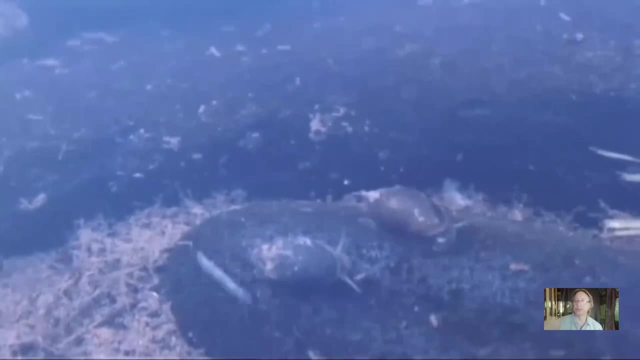 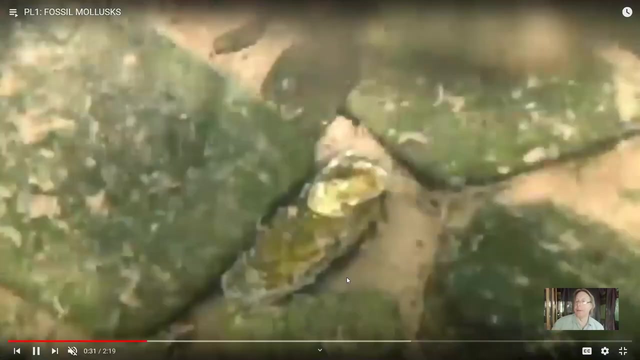 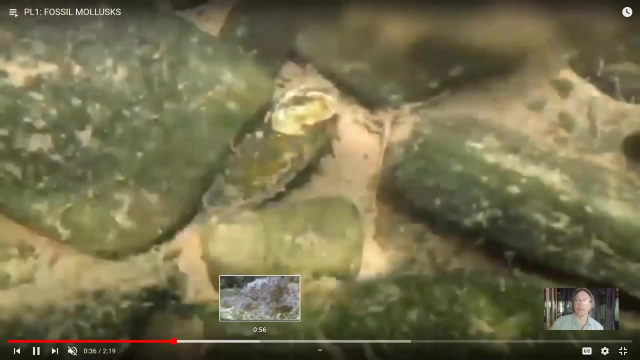 as clams, mussels, oysters, et cetera, but also then here's a little planarian- actually you can see in the background- but then also squid and octopi, all right, So mollusks are first known from the. 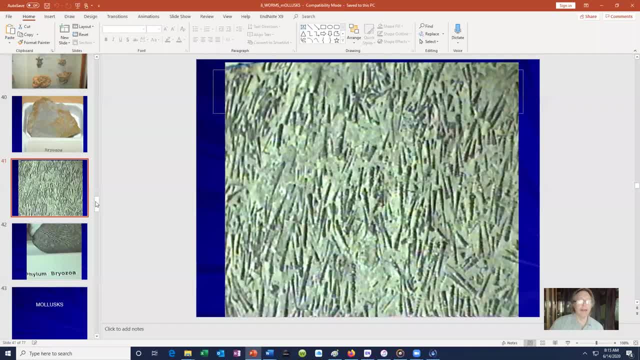 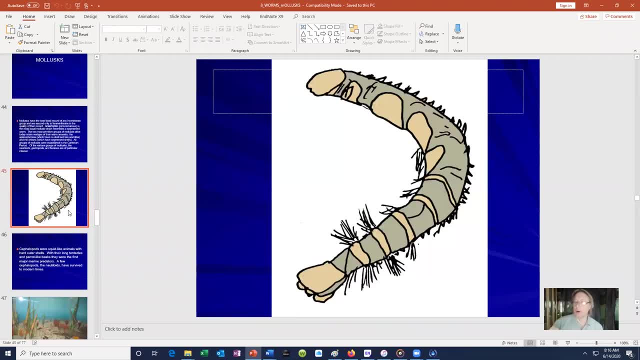 from the Cambrian period, although the Ediacaran animal, Kimberella, many have feel are mollusk-like, and there are animal embryos from the Ediacaran which seem to be mollusk-like. So mollusks, or maybe the ancestors of mollusks. 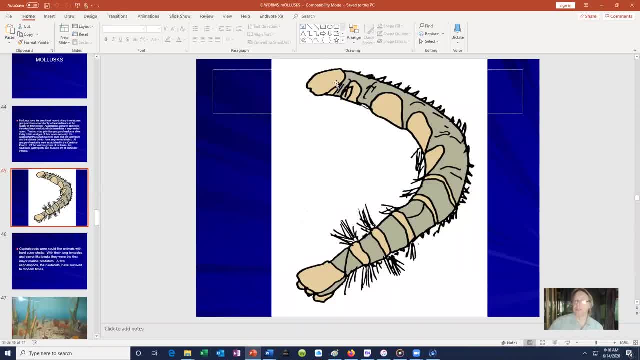 may have been present in the Ediacaran By the time we get to the Cambrian, we have mollusks which look like this. They look worm-like in their body. This is a canoplex, but it does have a shell. 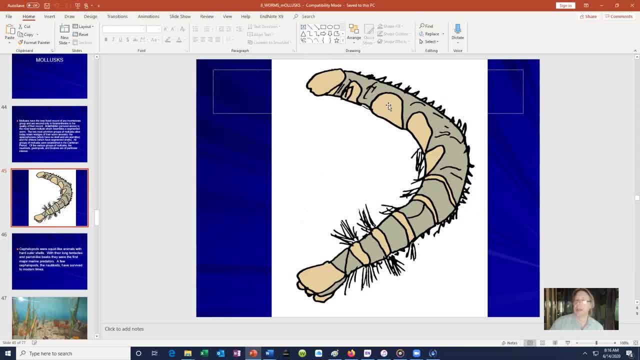 but notice that its shells come in segments. So here's a little piece of shell, here's a little piece of shell, a little piece of shell, et cetera. So this is a segmented animal which has little pieces of a segmented shell. unlike, say, a clam or a snail, Their shells aren't segmented. There are mollusks today, the most primitive mollusks, which do have segmented shells, such as chitons. So chitons are alive today. They have a segmented shell, which is how we think the first mollusks evolved from segmented worms. They developed a segmented shell In the earliest Cambrian. you don't have big fossils of animals. You have lots of little, tiny, hard fragments. 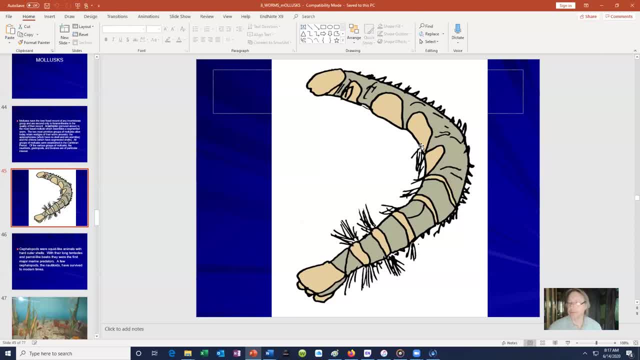 They're called SSFs- small shelly fossils- Although interestingly, I knew someone who looked at them, studied them and apparently among the people who studied them, SSFs. actually they're called SSFs. It means something else, but funny. 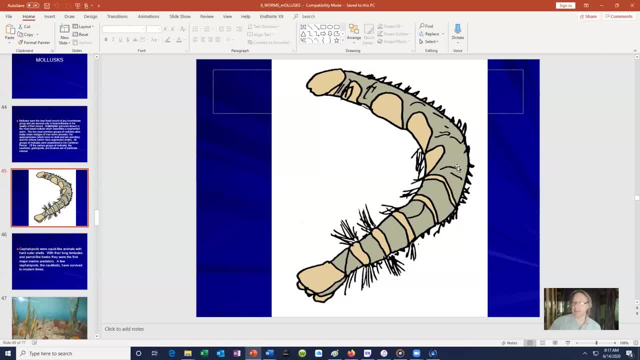 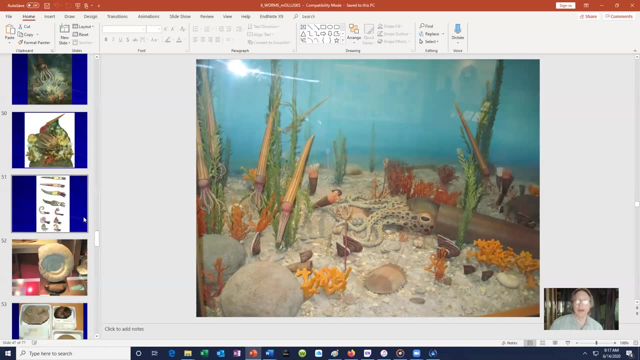 So mollusks evolved in stages and it seems that from segmented worms with small pieces of shell component that then larger, more complex mollusks would evolve. Now the one I would like to end with in the videos that I'll get back to in a second. 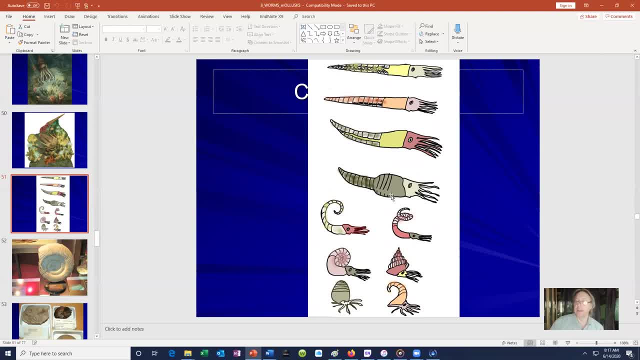 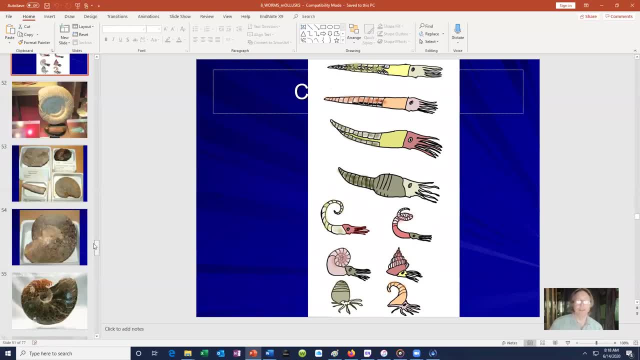 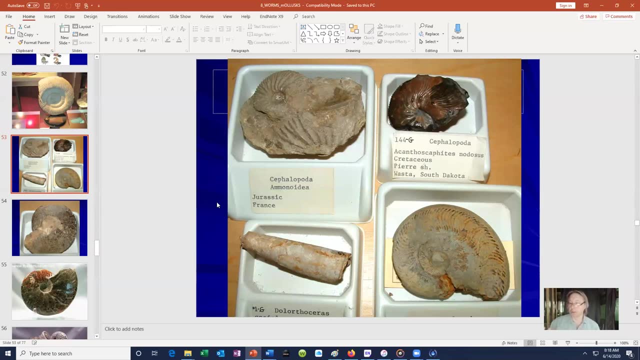 are the cephalopods. Now, today, the cephalopods are considered to include the octopi and squid, but in the Paleozoic, and then even going into the Mesozoic, there was an incredible diversity of armored squid relatives. 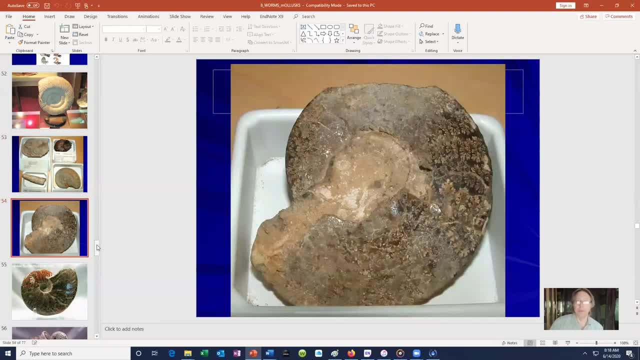 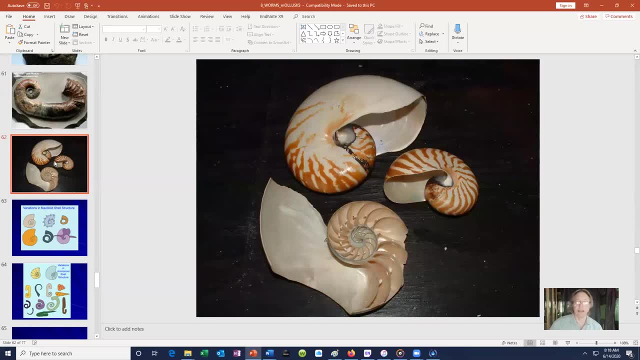 So they look like squid, but they had these shells around them, They could be huge, 10 feet long, some even 30 feet long. There is actually a relative of of. they're still alive today, So it is a squid-octopus relative, a cephalopod. 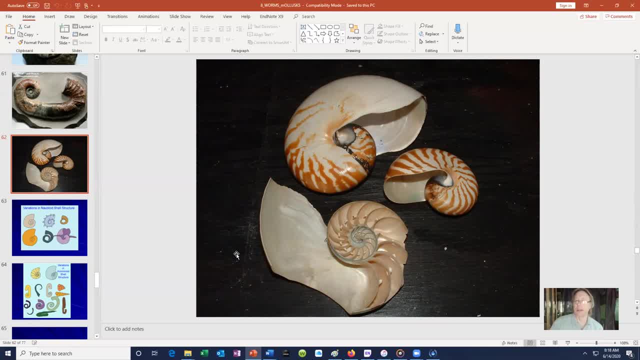 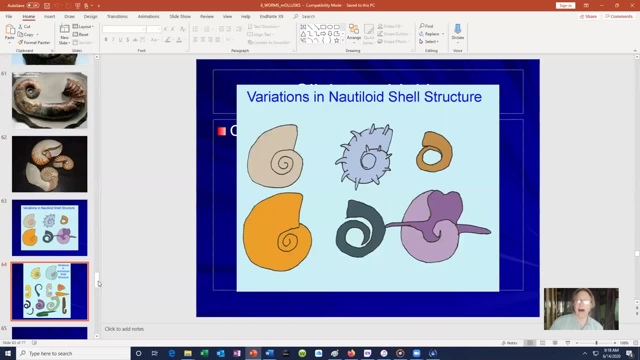 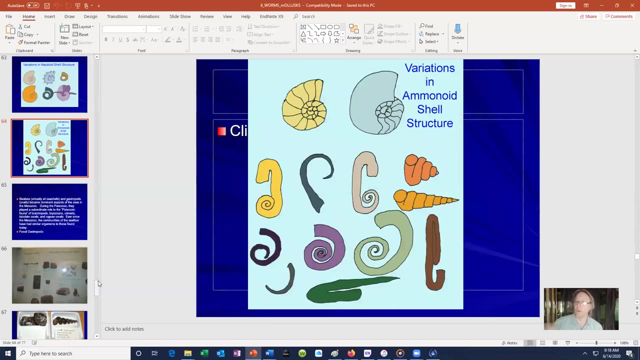 but it has a shell that it composes around itself, the nautilus, And there have been variations in the nautilus And when we think of the big marine reptiles of the Mesozoic, many of them were feeding on this group of armored cephalopods. 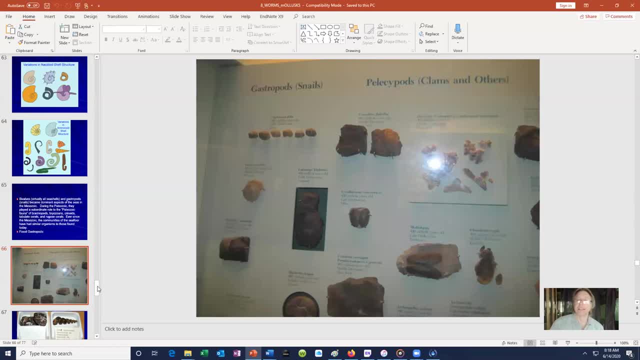 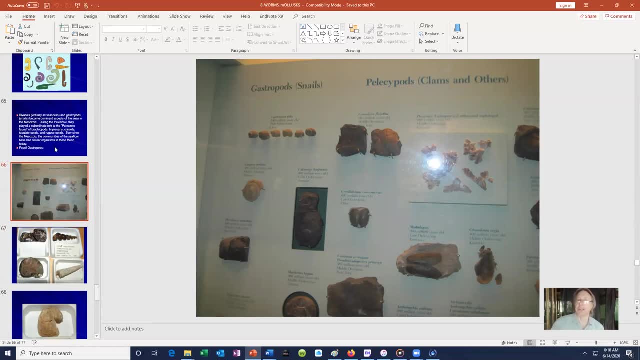 which were quite common. Now, mollusks not only include those you know, octopi and squid and the like, but then also many other members. Now, if the shell has only one component, then that's the most common group is what are called the gastropods. 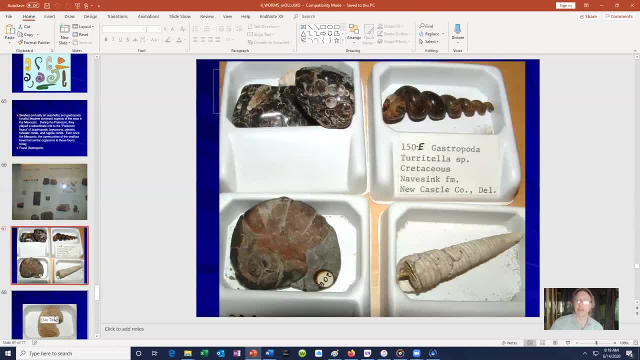 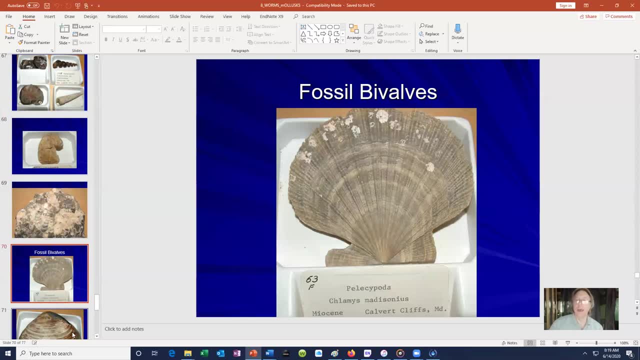 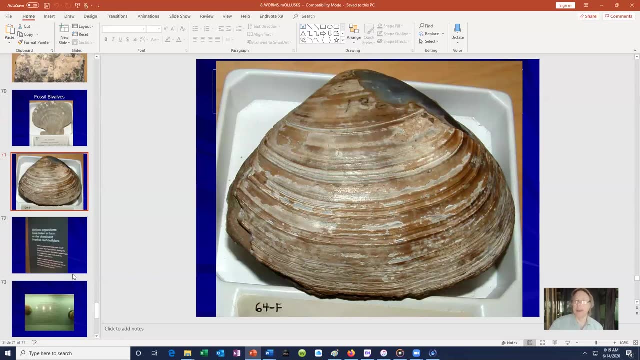 which includes snails. So notice, all of these shells have only one component. If, however, there are two halves, then it is known as a bivalve. All right, They have been important. They were important in the past, And so there were some bivalves, for example. 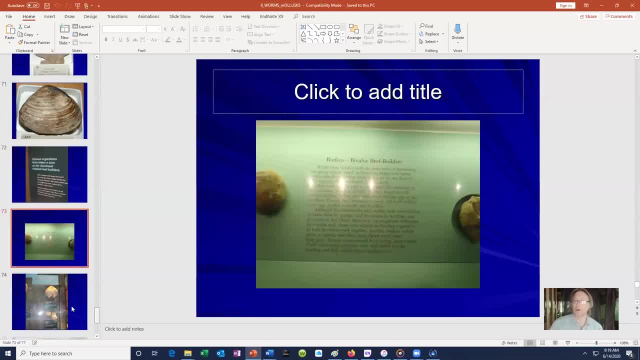 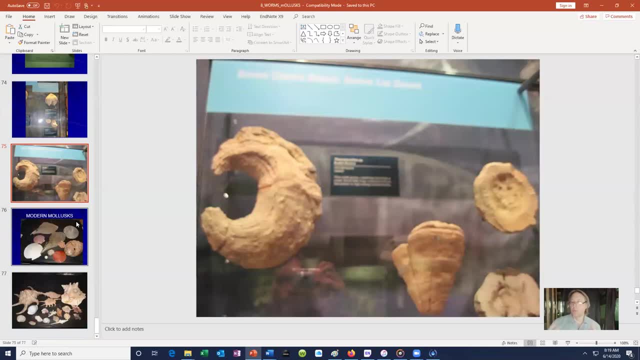 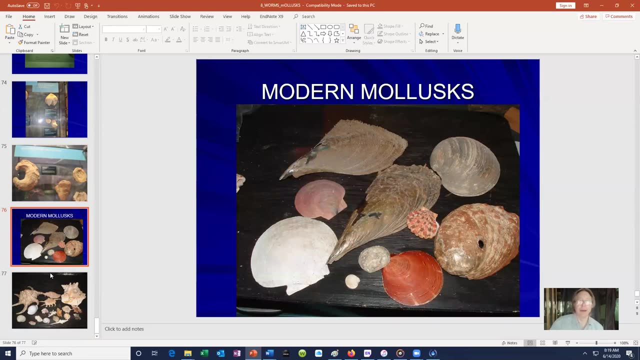 called the rudest clams, which were not only large but were significant reef builders, meaning that not only were these bivalves important in and of themselves, but if they were major components of reefs, then that would have made them important for all of the life on the sea floor. 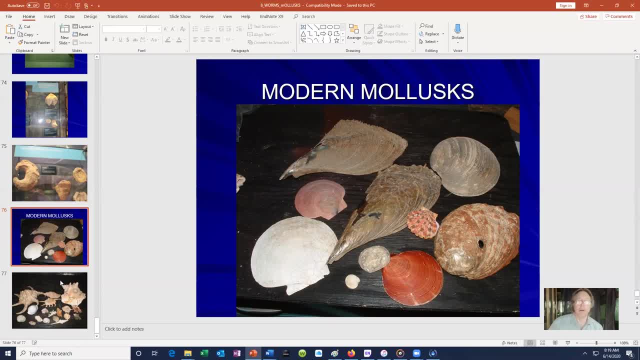 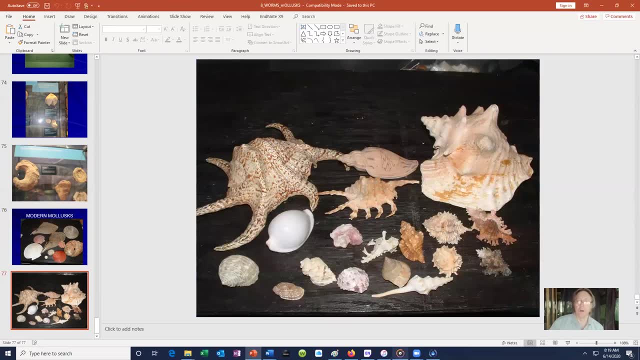 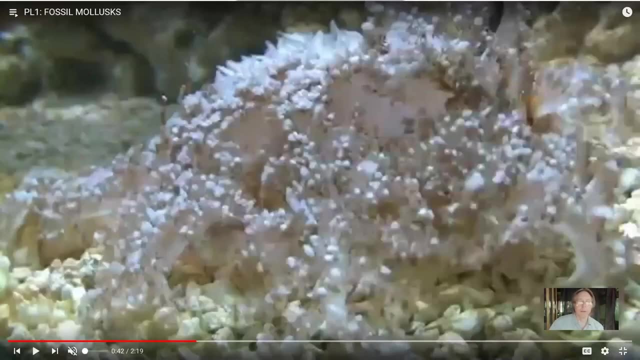 And so there are certainly, you know, modern mollusks which are bivalves and modern mollusks which are gastropods, with the one half of the shell, And there are other groups of mollusks as well. All right, 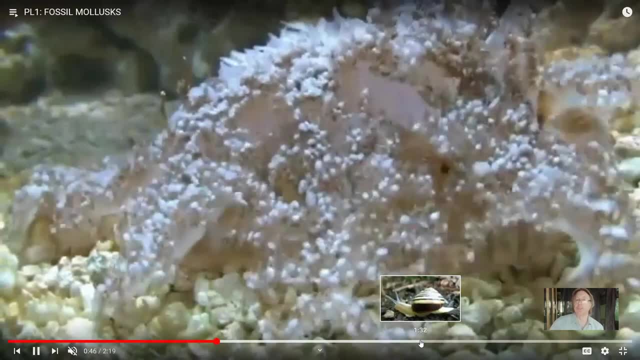 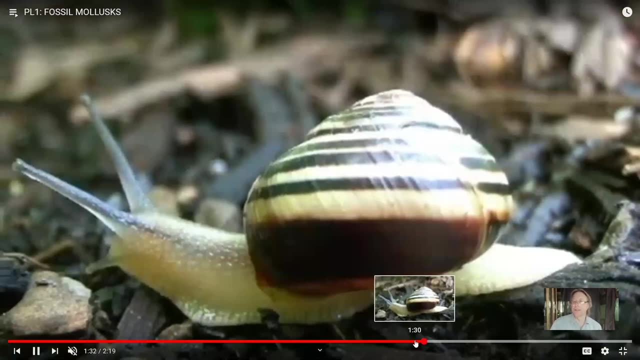 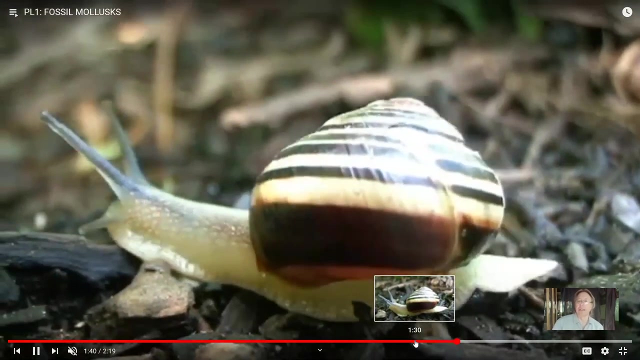 So here's a mollusk here, some of which have lost their shells, Some have come on to land. So, while mollusks are predominant, they are predominantly aquatic, being found in both marine and freshwater environments. Snails actually have been able to come on to land. 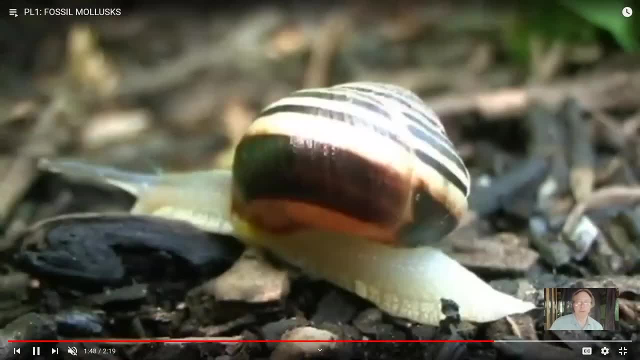 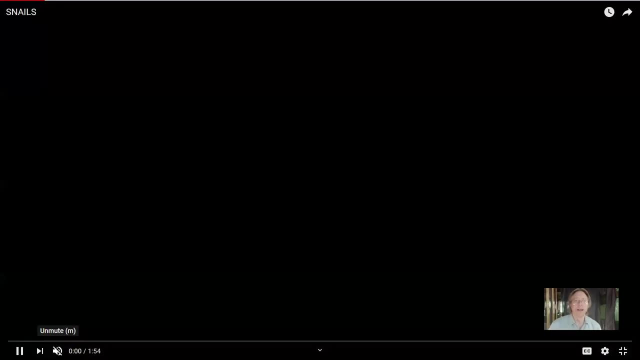 So I won't mention them further. But when we talk about terrestrial organisms, snails and slugs are certainly, you know, to be included among them, Although, once again, they are not. they are not a dominant, So you know. 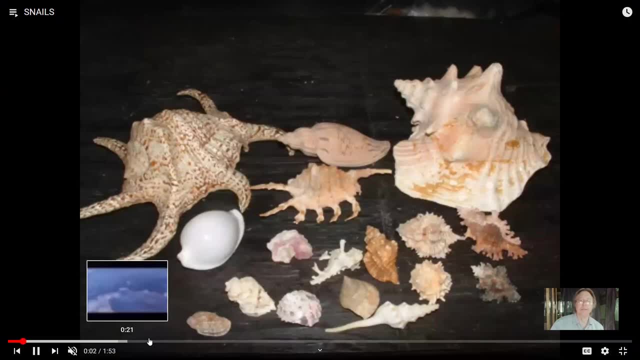 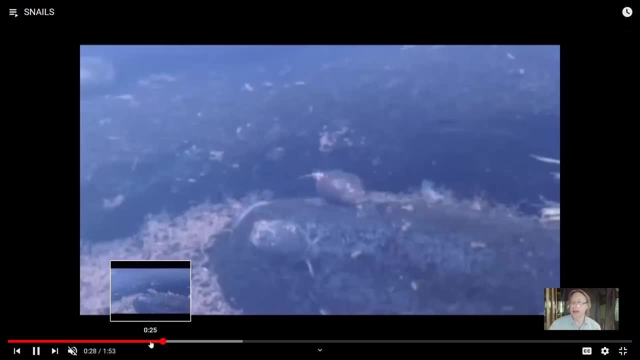 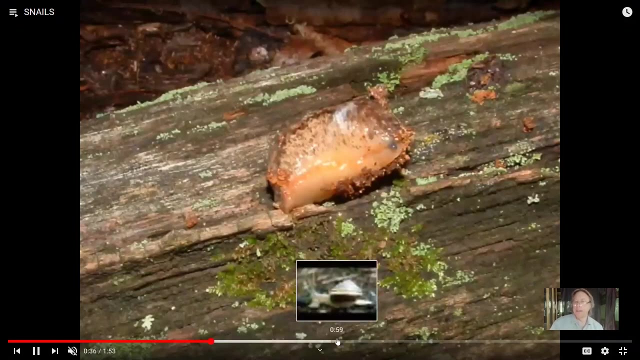 mollusks are a group of invertebrates And they are higher invertebrates. They are bilaterally symmetrical, but they do have a body cavity. They do have a heart and blood vessels. For most of them, the circulatory system is incomplete. 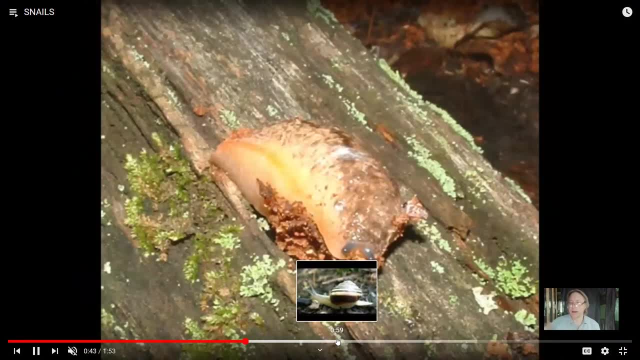 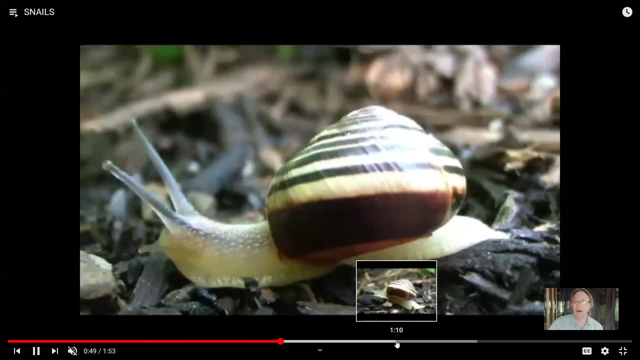 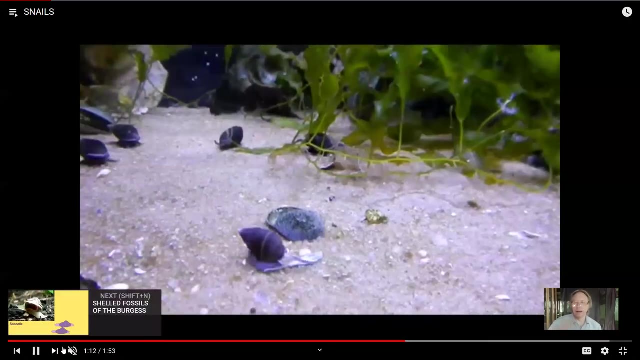 So the blood vessels end and the blood kind of leaks out into the body cavity and then finds its way back in. So they don't have they don't have a big strong heart, with the exception of things like octopi and squid which do have a closed circulatory system. 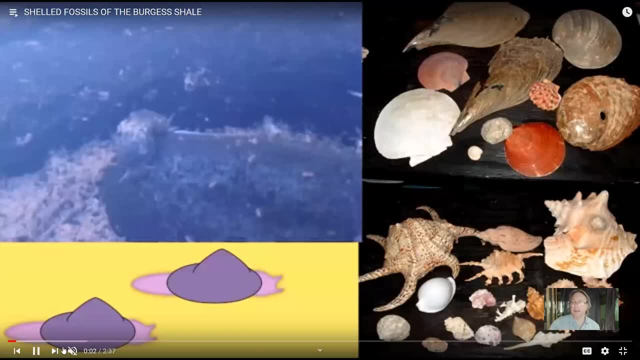 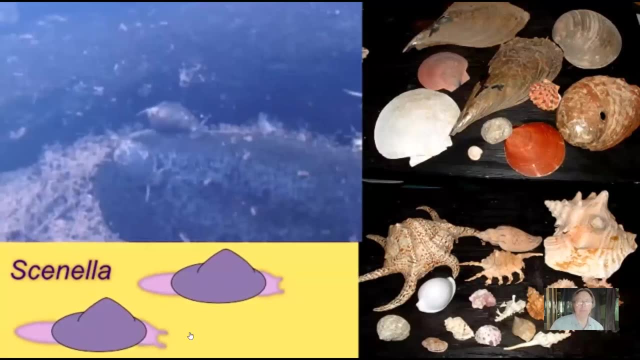 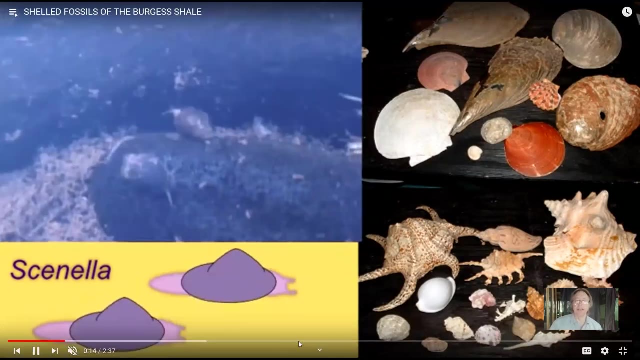 And in the Ediacaran period there are hints of mollusks or mollusk relatives, But certainly by the Cambrian. we know that mollusks diversify, So there are definitely shelled animals like these that are present in say. 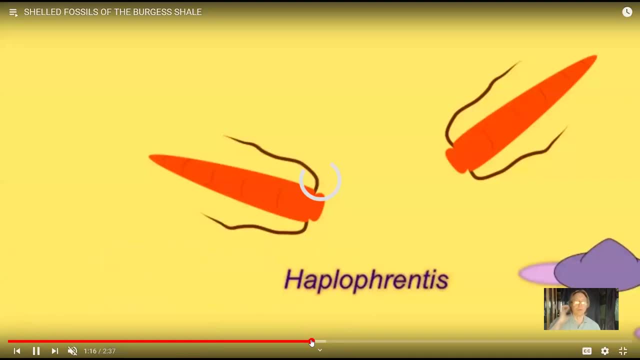 the Burgess Shale and some of the ones which you're about to see as well, And then at the very beginning of the Cambrian. once again, they're all of these little pieces of fossils, those small shelly fossils, which indicate that. 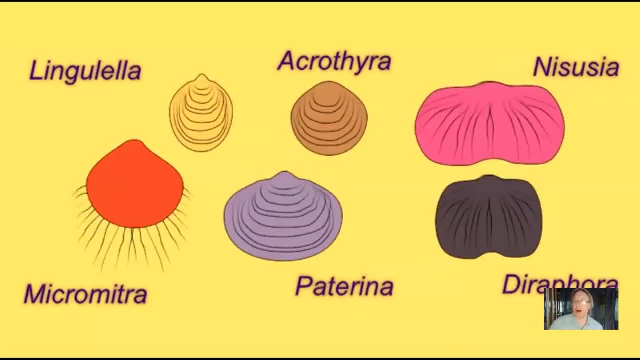 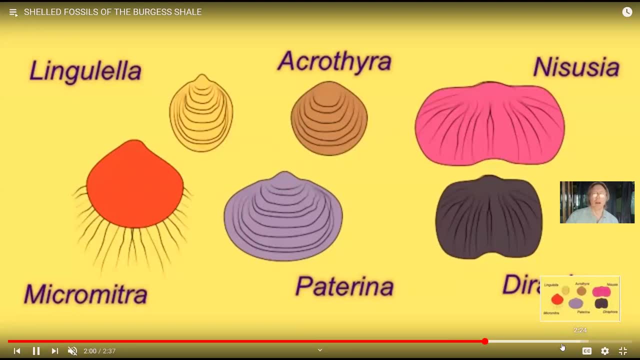 that mollusks were present. So mollusks are common today, And mollusks were common in the fossil era as well, And so, once again, here are some of the fossils of the Cambrian. Now, these animals have a very good fossil record. 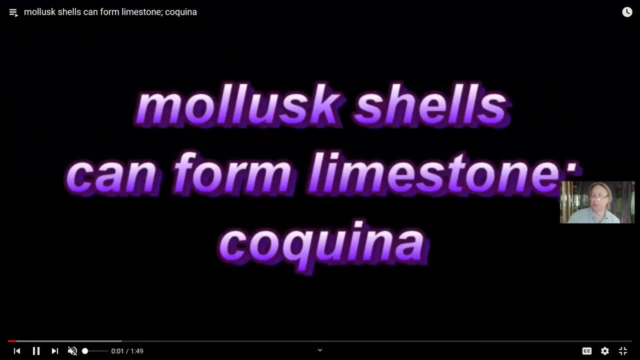 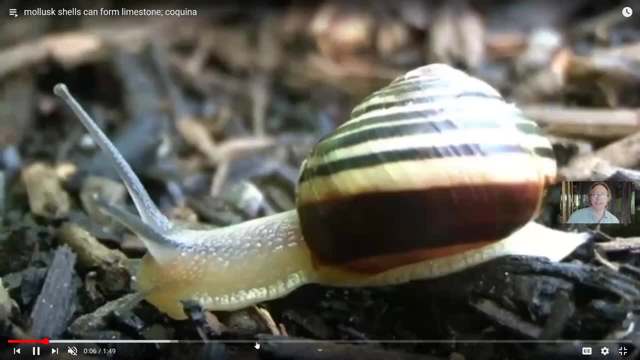 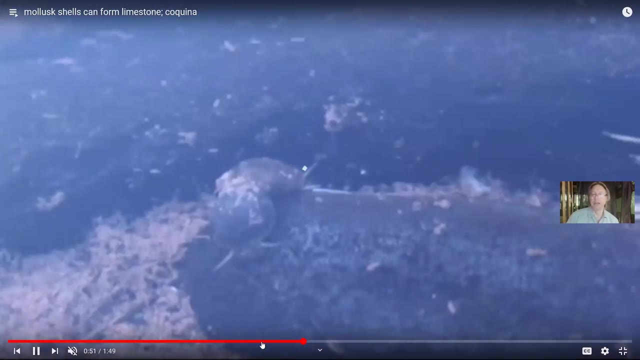 Obviously, their shells would preserve rather well. In fact, there's a type of limestone called coquina, which is then predominantly, predominantly, made of mollusk shells, Although this could be bivalves, it could be snails, it could be those armored. 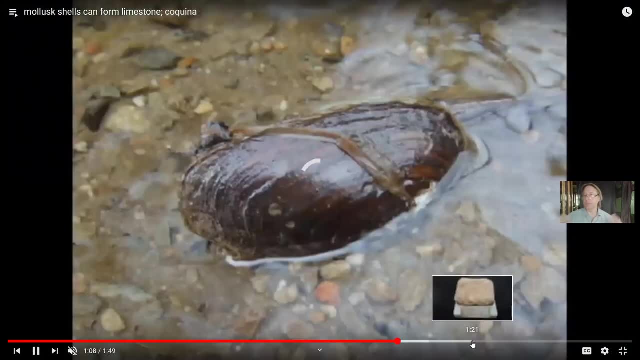 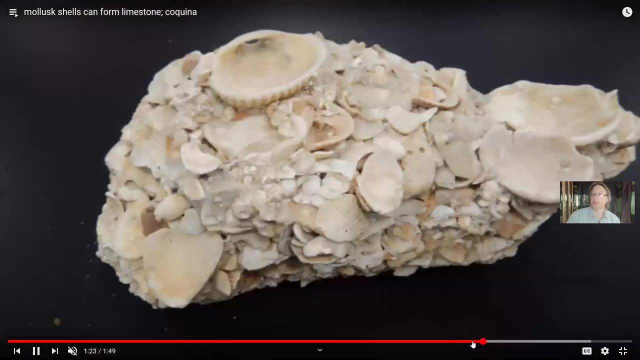 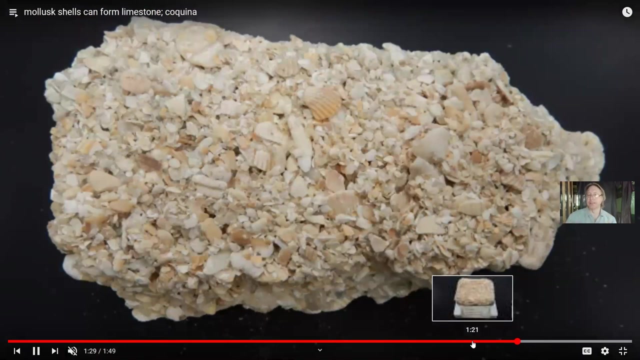 it could be those armored squid. There are different animals which make calcium carbonate, even microscopic animals that could contribute to limestone, But some limestone is primarily composed of the shells of mollusks, And so this is called coquina, And so this improves our ability to study. 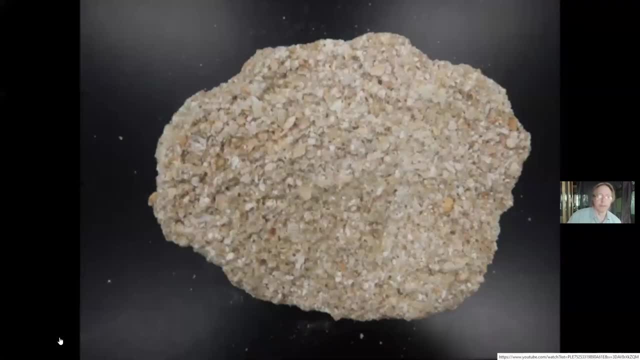 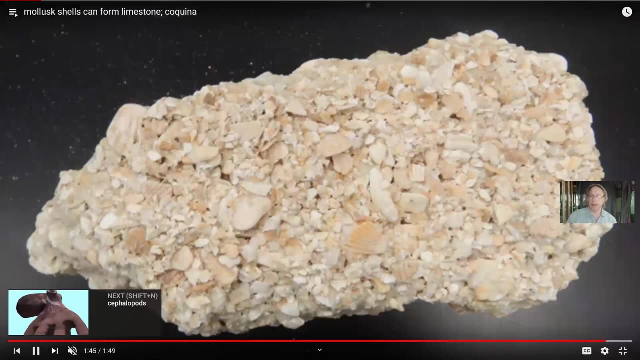 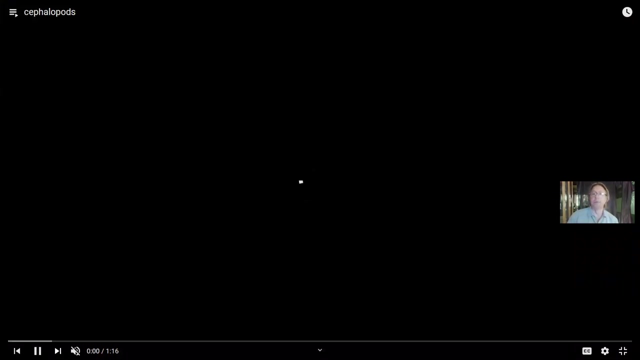 you know their fossils because of you know the, their hard parts, which are then likely to fossilize Now cephalopods. they have greatly modified the molluscan body plan. The modern ones have greatly reduced their shell. 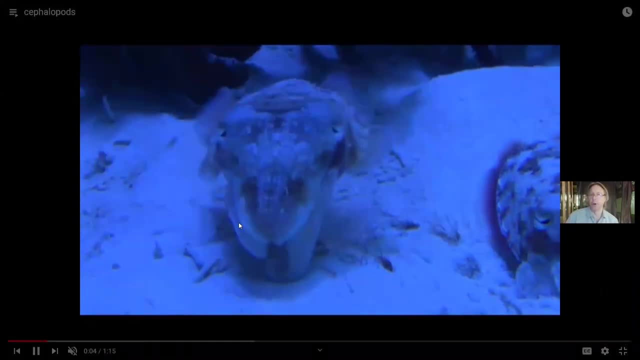 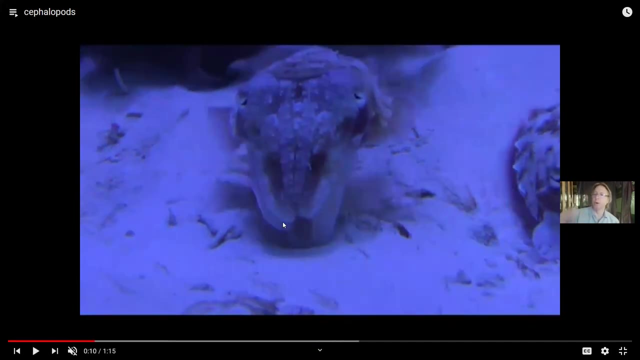 So we have squid, we have octopi, and these are cuttlefish also in the cephalopod group. Mollusks have a foot All right, And so in a clam the foot is what just can burrow. 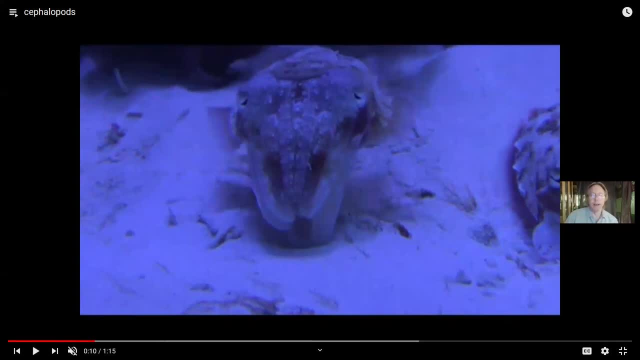 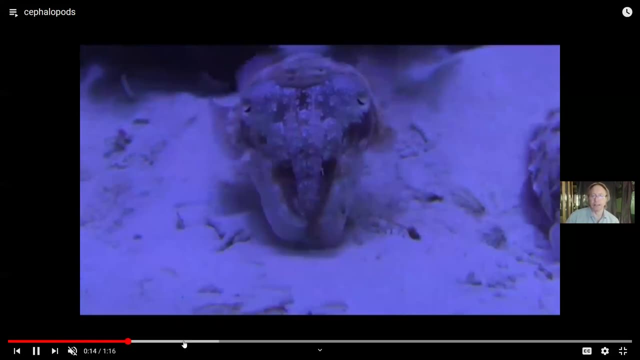 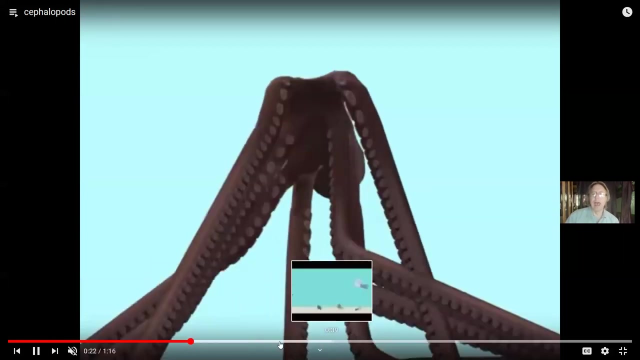 And it's just this one single structure, Whereas in the octopi, squid and cuttlefish it can be divided into separate tentacles. All right, And so they have clearly modified the molluscan body plan, And these are an ancient group. 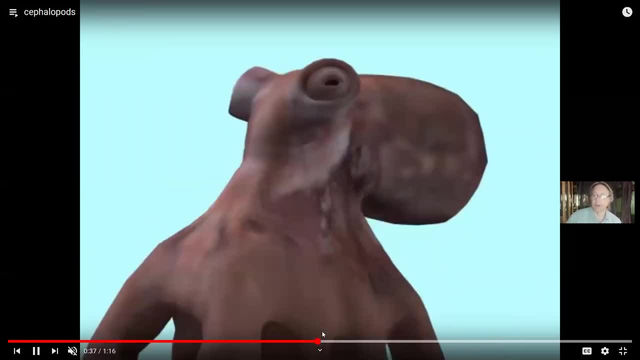 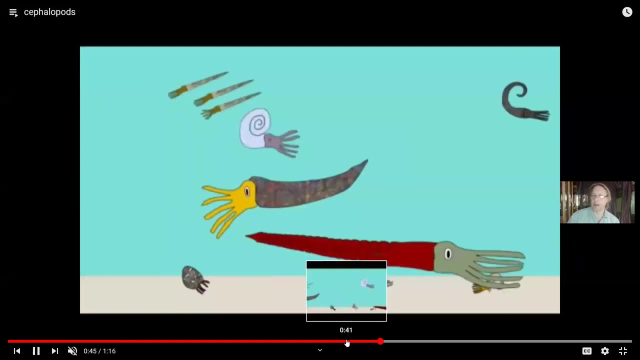 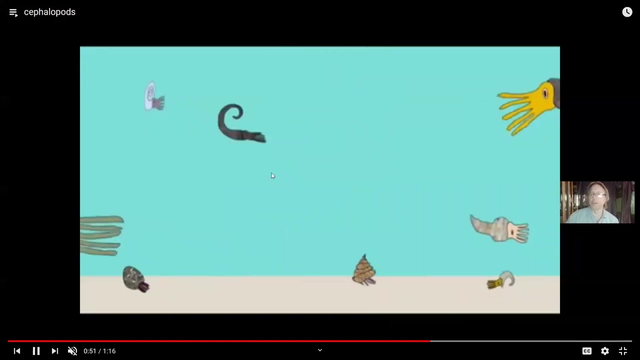 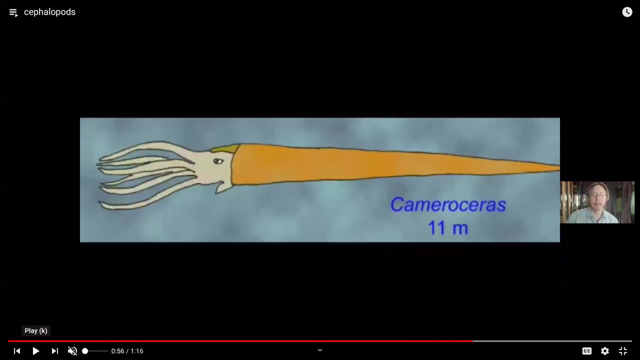 which were extremely successful in the fossil record. So by the Ordovician period there was this great diversity of armored cephalopods. Some had straight shells, Some had curled shells, Some were small and would have been a bottom dwelling. This one might have reached more than 30 feet in length. 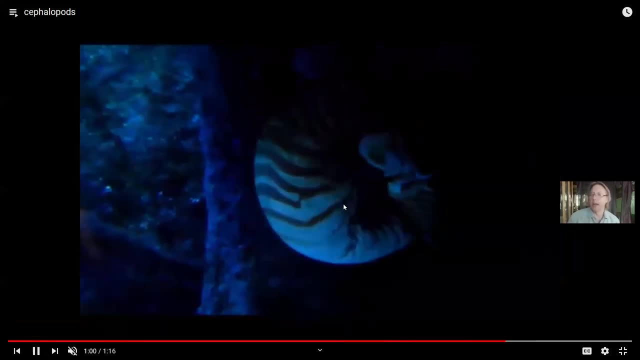 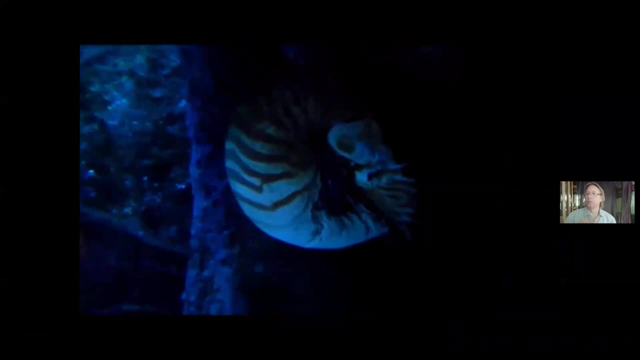 And then here is the Nautilus. It is the only shelled cephalopod which remains today, And so, while the shelled cephalopods were incredibly diverse, such as the ammonites which existed in the Mesozoic, 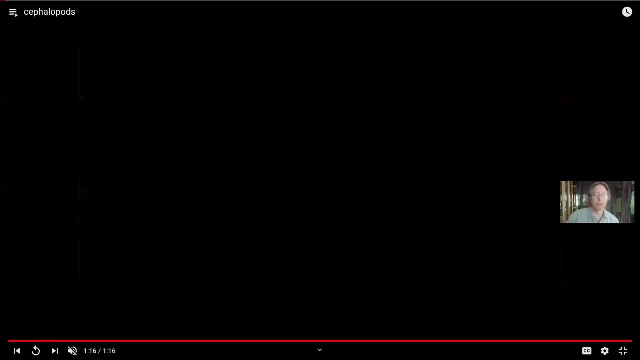 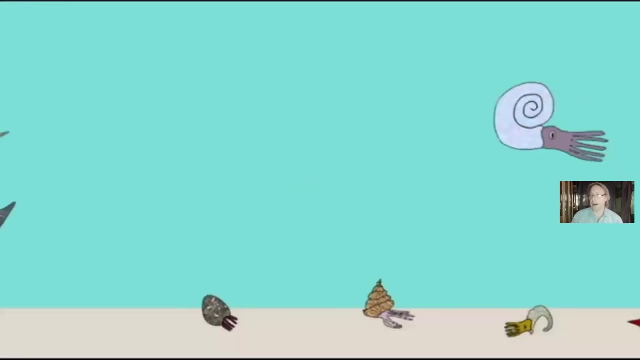 this is the only lineage which has survived until today. So a challenge is that invertebrates are so much more varied than what most people appreciate today. I mean, there are so many different kinds of invertebrates. And then if we were to include fossil invertebrates, 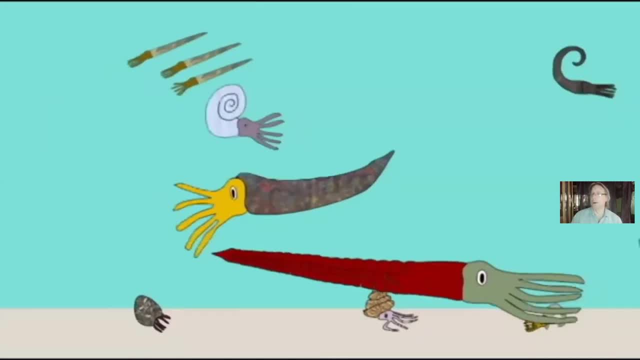 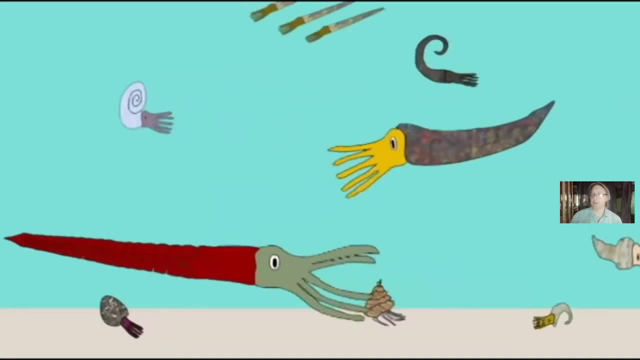 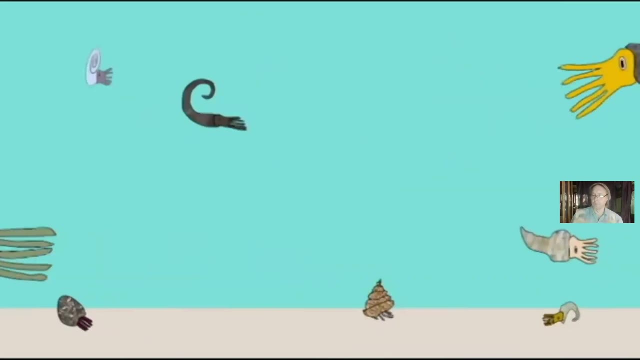 you know that would be even more the case. What I hoped to do here was just to introduce a number of different invertebrate groups to get across the idea of the diversity, Also a bit of the history, where the foundations of many of the branches were laid down in the Ediacaran period.